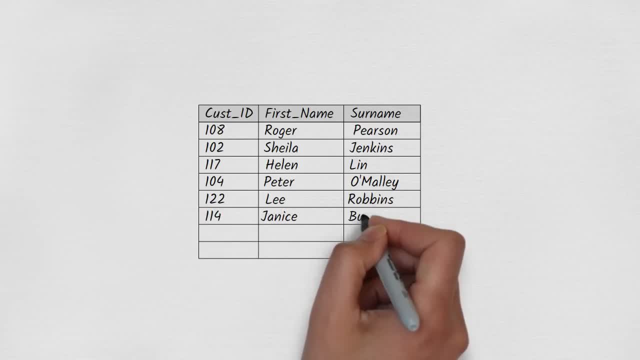 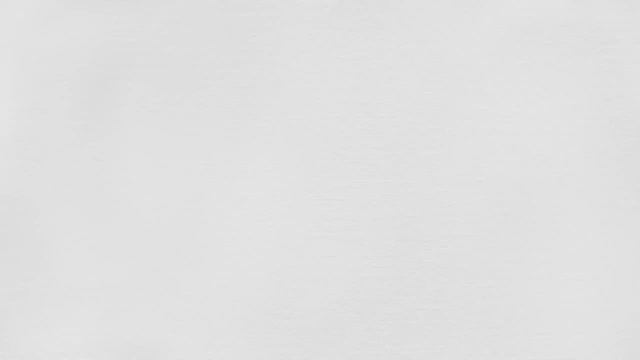 practical perspective. We'll keep the jargon to a minimum and we'll use lots of examples as we go. By the end of it, you'll understand the so-called normal forms, from first normal form all the way up to fifth normal form, and you'll have a clear sense of what 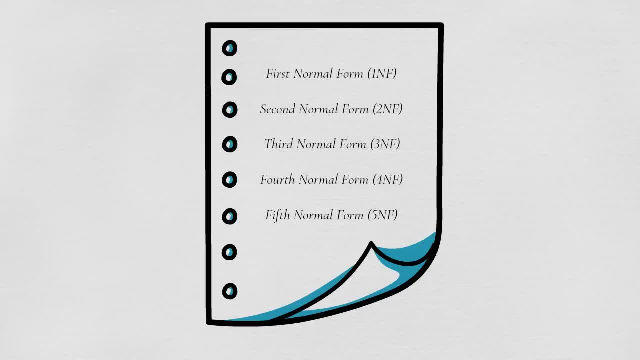 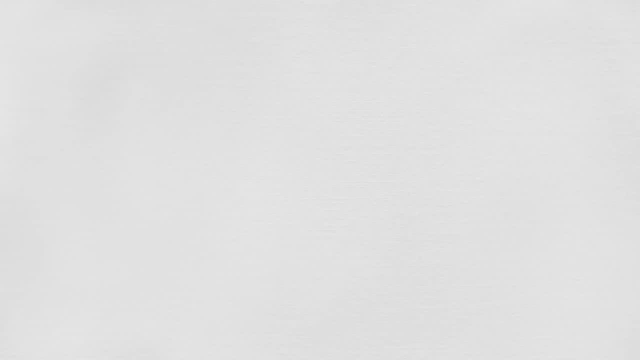 we gain by doing normalization and what we lose by failing to do it. This is Decomplexify, bringing a welcome dose of simplicity to complex topics. Data: It's everywhere And some of it is wrong. By and large, even if you understand the definition of a problem, it's nothing but a aquesta problem. 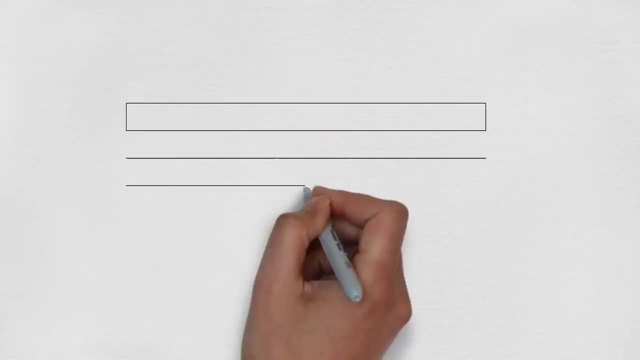 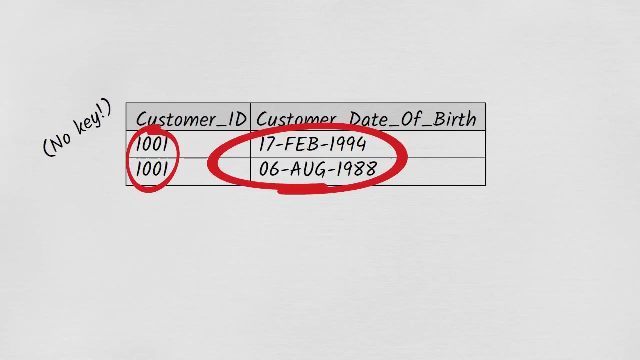 a good database design can't protect against bad data, But there are some cases of bad data that a good database design can protect against. These are cases where the data is telling us something that logically cannot possibly be true. One customer with two dates of birth is 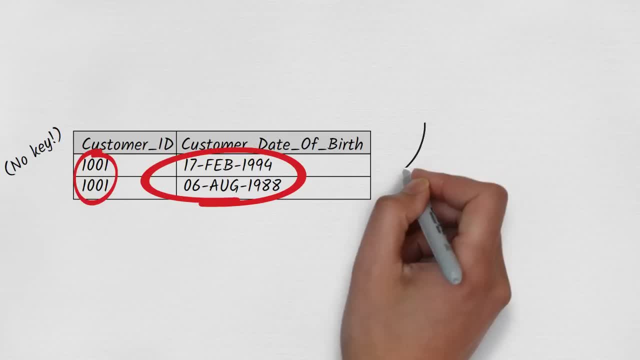 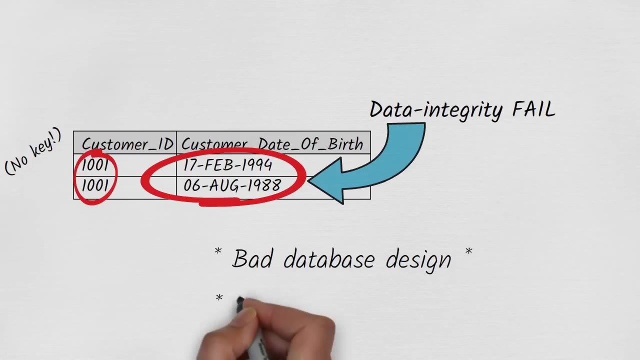 logically impossible. It's what we might call a failure of data integrity. The data can't be trusted because it disagrees with itself. When data disagrees with itself, that's more than just a problem of bad data. It's a problem of bad database design. Specifically, 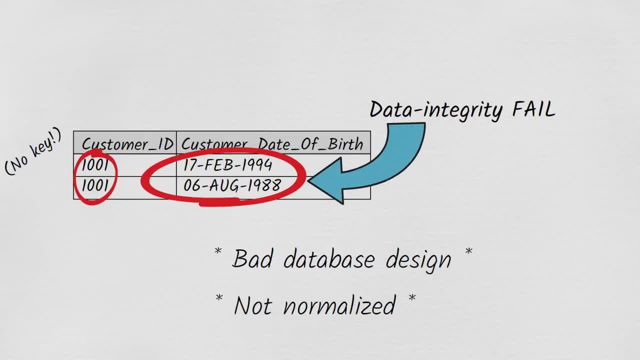 it's what happens when a database design isn't properly normalized. So what does normalization mean? When you normalize a database table, you structure it in such a way that it can't express redundant information. So, for example, in a normalized table you wouldn't be able to give customer 1001 two dates of birth, even if you wanted to. 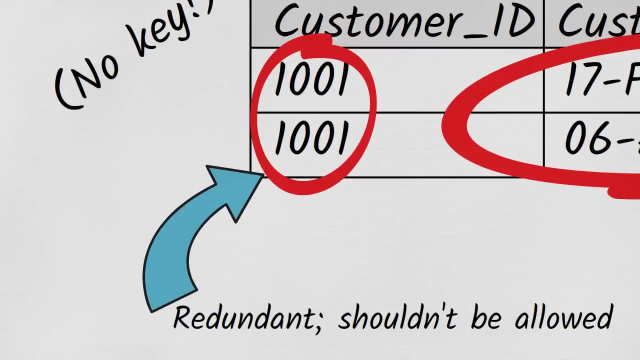 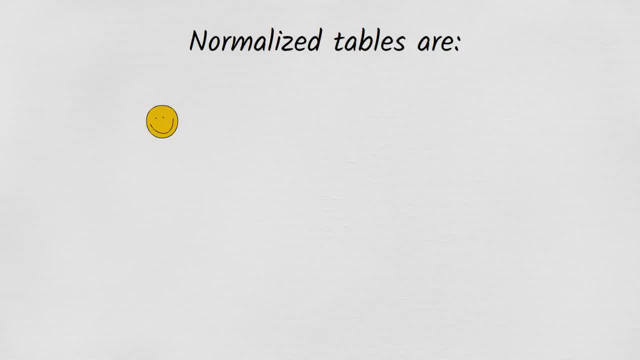 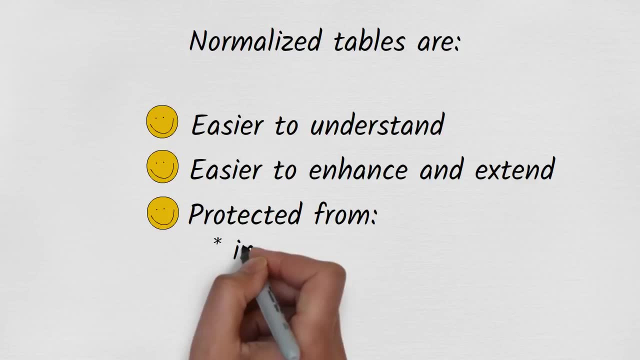 Very broadly. the table can only express one version of the truth. Normalized tables are not only protected from contradictory data, they're also easier to understand, easier to enhance and extend, and protected from insertion anomalies, update anomalies and deletion anomalies. More on these. 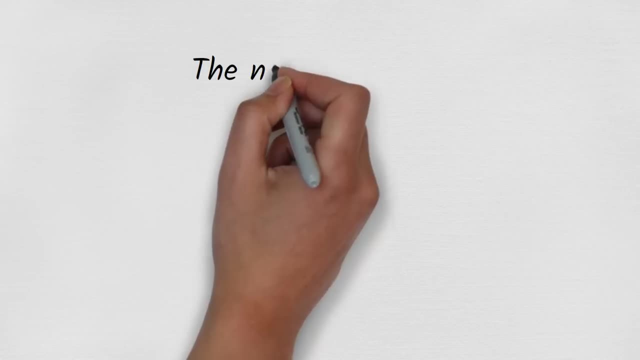 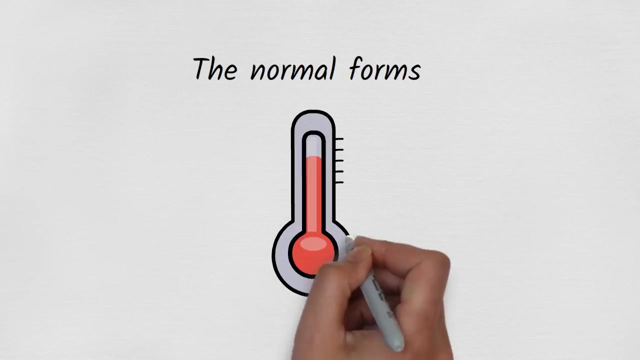 later. How do we determine whether a table isn't normalized enough? In other words, how do we determine if there's a danger that redundant data could creep into the table? Well, it turns out that there are sets of criteria we can use to assess the level of danger. 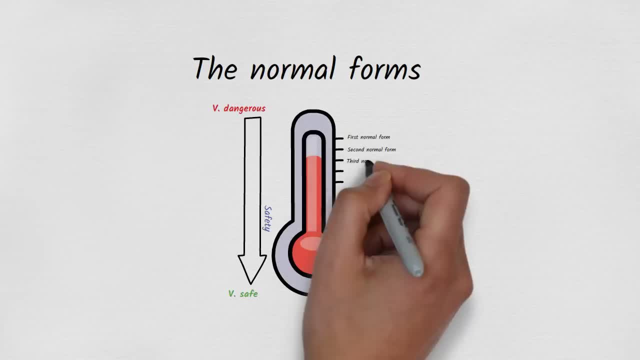 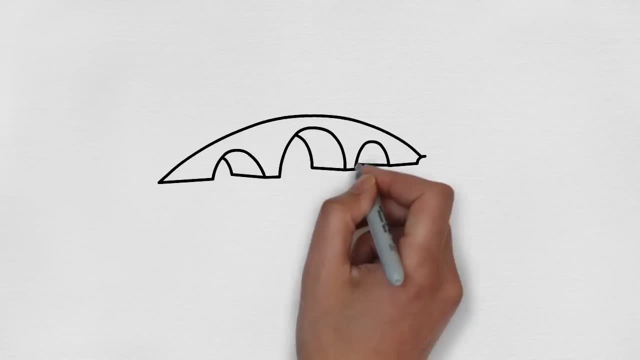 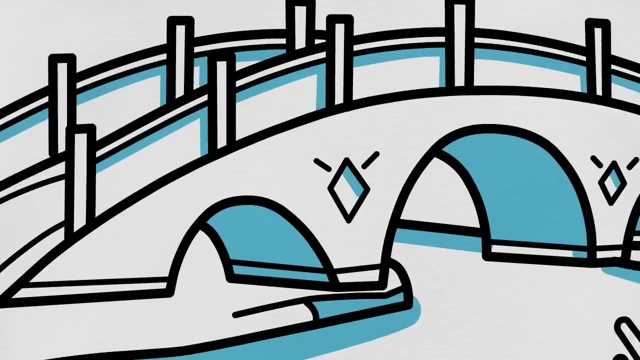 These sets of criteria have names like first, normal form, second, normal form, third, normal form, and so on. Think of these normal forms by analogy to safety assessments. We might imagine an engineer doing a very basic safety assessment on a bridge. Let's say the bridge passes the basic assessment, which means it achieves safety level one, safe for. 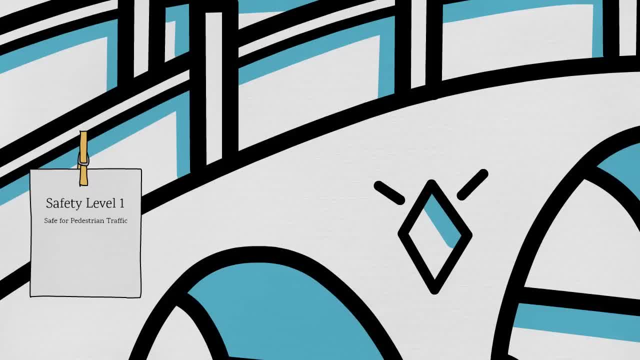 pedestrian traffic. That gives us some comfort, but suppose we want to know if cars can safely drive across the bridge. To answer that question, we need the engineer to perform an even stricter assessment of the bridge. Let's imagine that the engineer goes ahead and does the stricter. 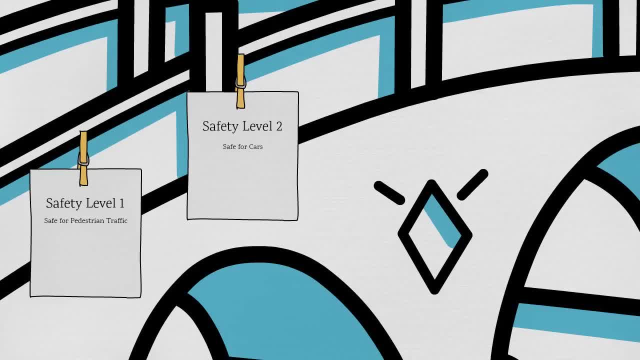 assessment and then we can use the bridge to assess the level of danger And again the bridge passes, achieving safety level two, safe for cars. If even this doesn't satisfy us, we might ask the engineer to assess the bridge for safety level three, safe for trucks, and so on. 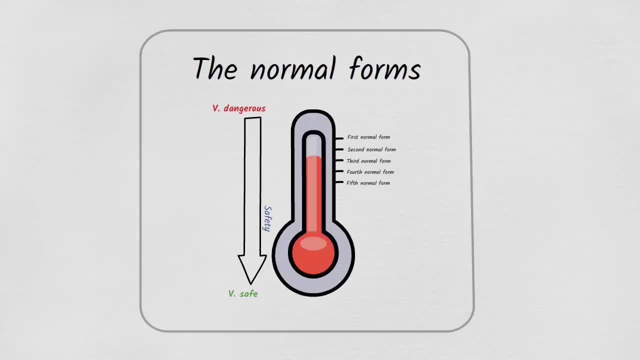 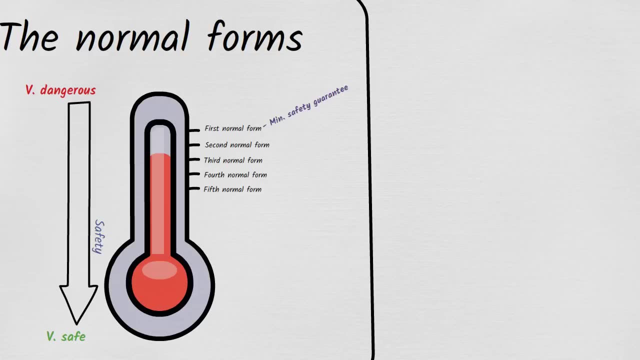 The normal forms of database theory work the same way. If we discover that a table meets the requirements of first normal form, that's a bare minimum safety guarantee. If we further discover that the table meets the requirements of second normal form, that's an even greater safety guarantee, And so on. 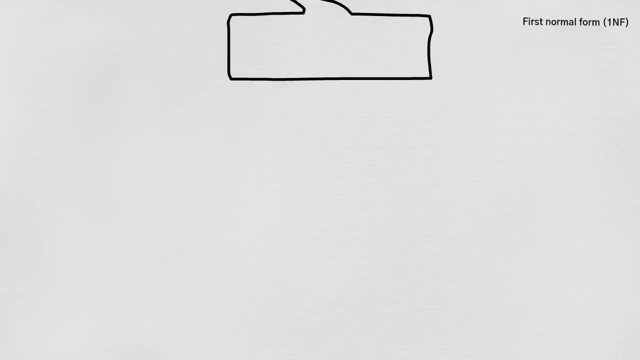 So let's begin at the beginning with first normal form. Suppose you and I are both confronted by this question, You might answer John, Paul, George and Ringo. I might answer Paul, John, Ringo and George. Of course, my answer and your answer are equivalent. 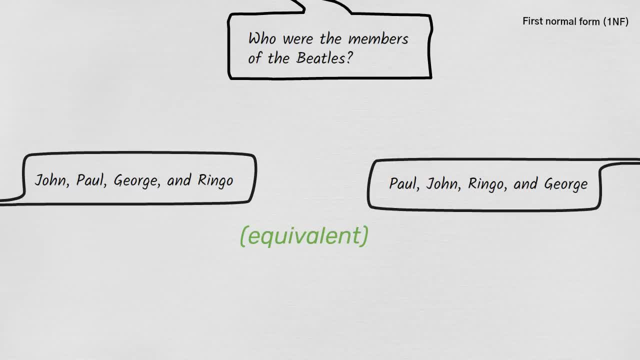 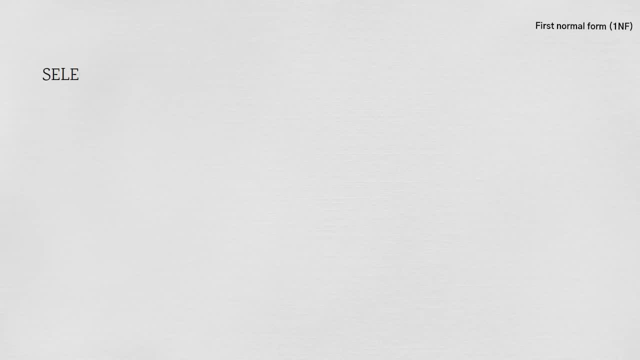 despite having the names in a different order. When it comes to relational databases, the same principle applies. Let's record the names of the Beatles in a table and then let's ask the database to return those names back to us. The results will get returned to us in an arbitrary order. For example, 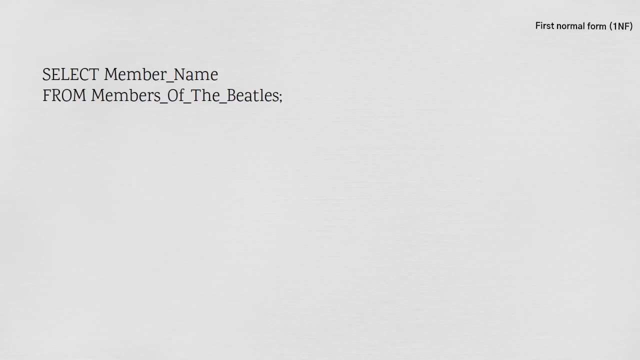 they might get returned like this or like this or in any other order. There is no right order. Are there ever situations where there's a right order? Suppose we write down the member's of the Beatles from tallest to shortest, like this: 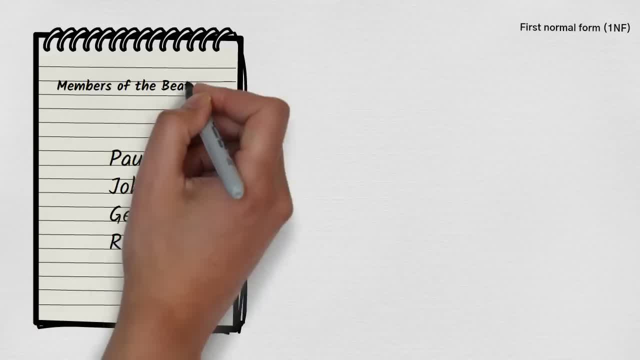 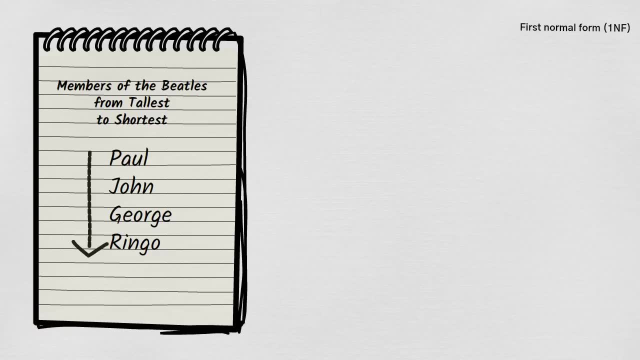 We title our list Members of the Beatles from Tallest to Shortest. In this list, it's not just the names that convey meaning. The order of the names conveys meaning too. Paul is the tallest, John is the second tallest, and so on. Lists like this are totally. 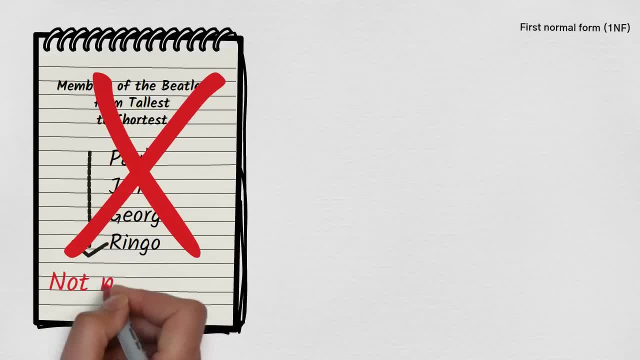 comprehensible to us, but they're not normalized. Remember, there's no such thing as row order within a relational database. So here we have our first violation of first normal form. When we use row order to convey information, we're violating first normal form. 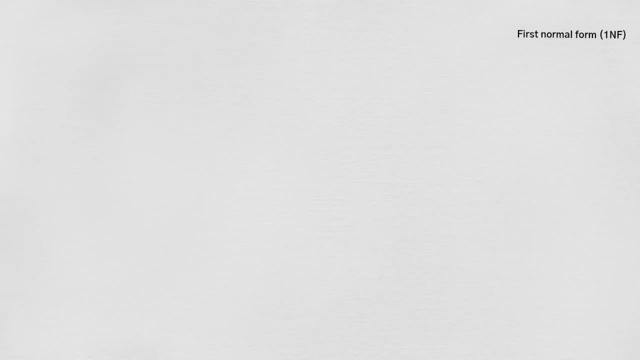 The solution is very simple. Be explicit. If we want to capture height information, we should devote a separate column to it. like this Or, even better, like this: So far, we've seen one way in which a design can fail to achieve first normal form. 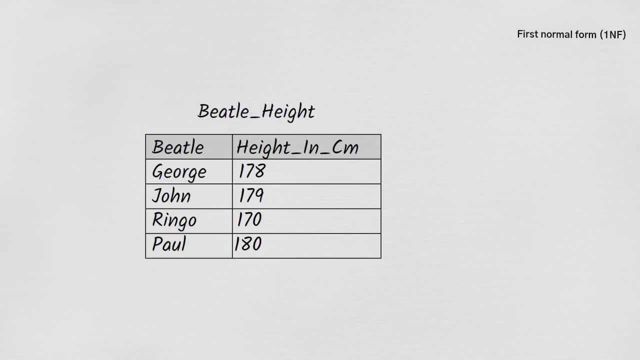 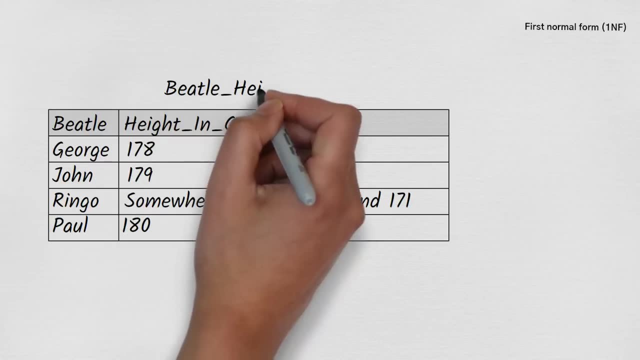 but there are others. A second way of violating first normal form involves mixing data types. Suppose our Beatle height dataset looked like this: If you're accustomed to spreadsheets, you'll be aware that they typically won't stop you from having more than one data type within a single column, For example. 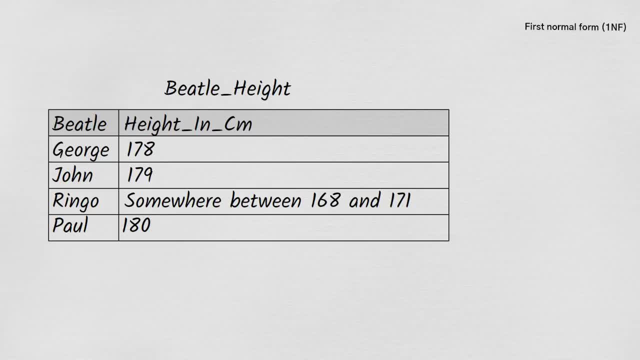 they won't stop you from storing both numbers and strings in a column, But in a relational database you're not allowed to be cagey or ambiguous about a column's data type: the values that go in the height in centimeters. column can't be a mix of integers and strings. 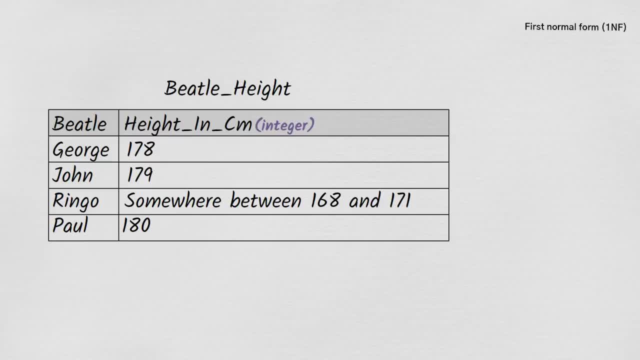 Once you define height in centimeters as being an integer column, then every value that goes into that column will be an integer: No strings, no timestamps, no data types of any kind other than integers. So mixing data types within a column is a violation of first normal form. 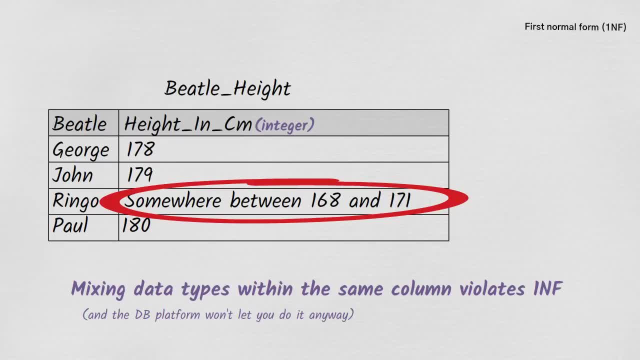 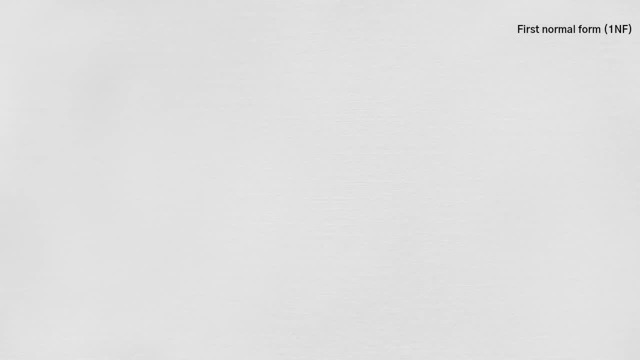 and in fact, the database platform won't even let you do it. A third way of violating first normal form is by designing a table without a primary key. A primary key is a column or a combination of columns that uniquely identifies a row in the 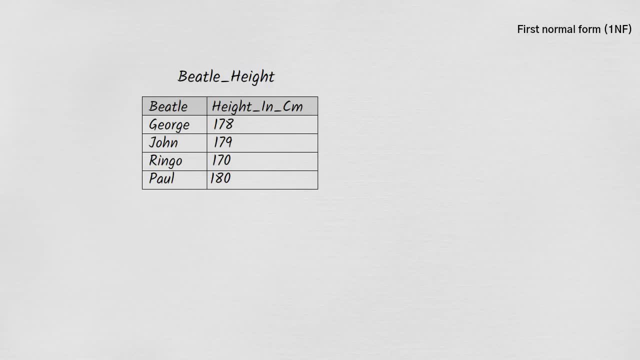 table. For example, in the table beetle height, our intention is that each row should tell us about one particular beetle, so we ought to designate beetle as the primary key of the beetle height table. The database platform will need to know about our choice of primary key when. 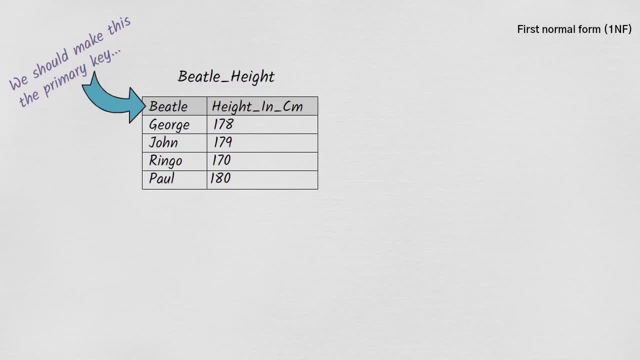 designing the first normal form, the primary key. so we'll want to get the primary key into the database. by doing something like this, With the primary key in place, the database platform will prevent multiple rows for the same beetle from ever being inserted. That's a good thing, because multiple rows for the 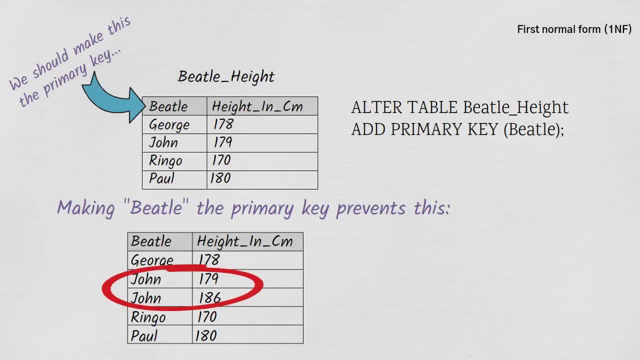 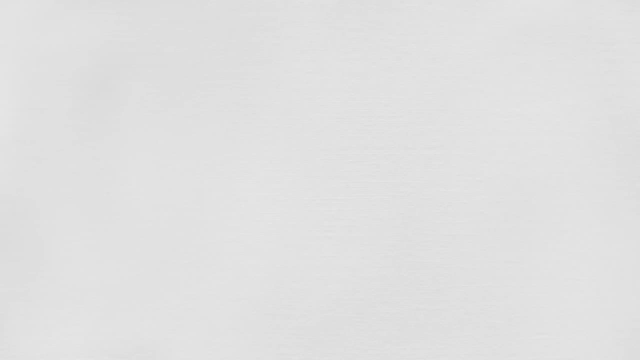 same beetle would be nonsensical and perhaps contradictory. Obviously, a beetle can't have two different heights at once. Every table we design should have a primary key. If it doesn't, it's not in first normal form. The last way of failing to achieve first normal form involves the notion of repeating groups. 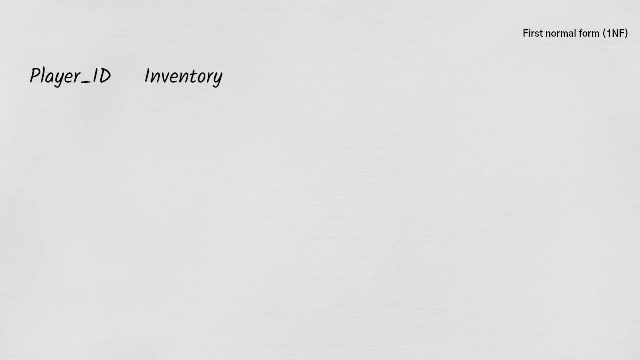 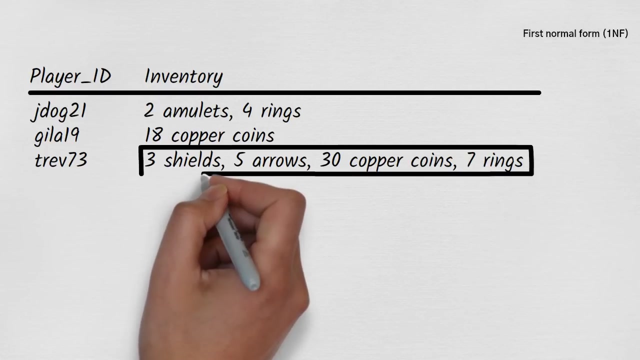 Suppose we're designing a database for an online multiplayer game. At a given time, each player has a number of items of different types like arrows, shields and copper coins. We might represent the situation like this: A player's inventory is what we call a repeating group. 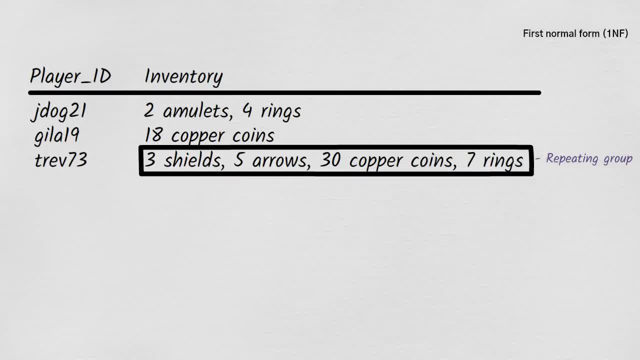 Each inventory contains potentially many different types of items – arrows, shields, copper coins and so on, And in fact there may be hundreds of different types of items that a player might have in their inventory. We could design a database table that represents the inventory as a string of text. 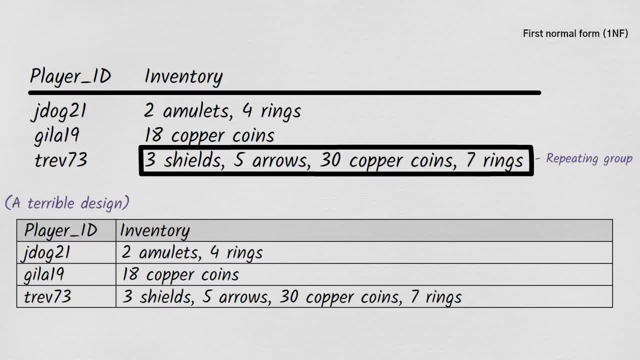 But this is a terrible design because there's no easy way of querying it. For example, if we want to know which players currently have more than ten copper coins, then having the inventory data lumped together in a text string will make it very impractical to write. 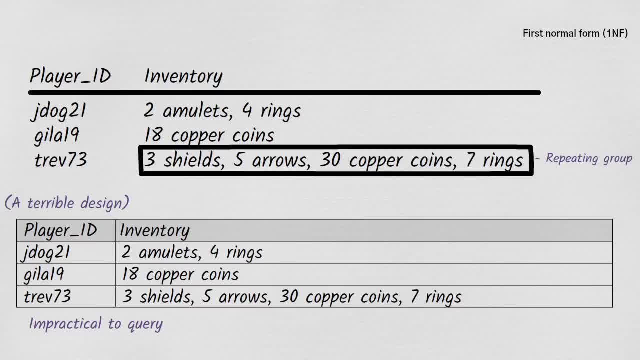 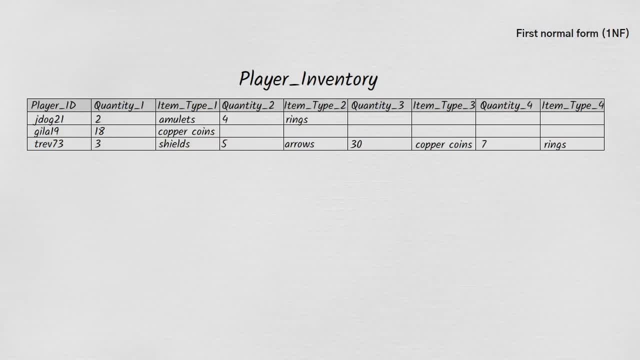 a query that gives us the answer. We might be tempted to represent the data like this: This lets us record up to four items per inventory, But given that a player can have an inventory consisting of hundreds of different types of items, how practical is it going to be to design a table with hundreds of columns? 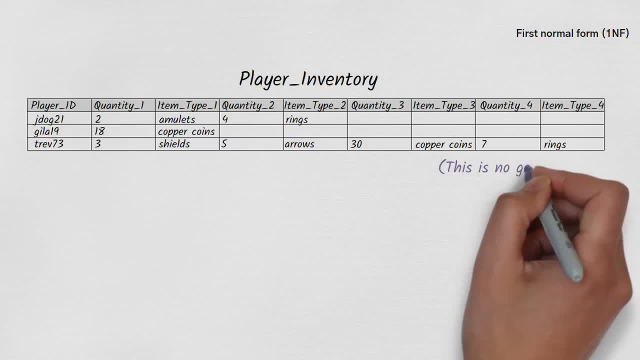 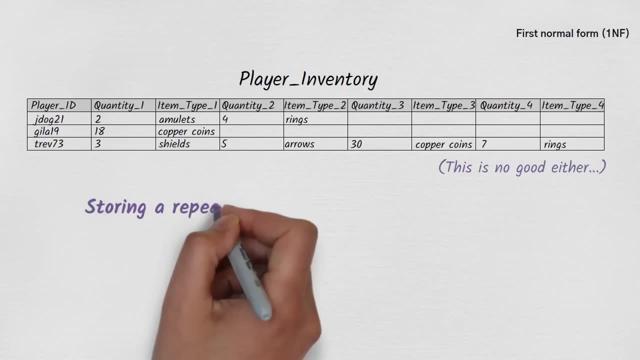 Even if we were to go ahead and create a super wide table to hold all possible inventory data querying, it would still be extremely awkward. The bottom line is that storing a repeating group of data items on a single row violates first normal form. So what sort of alternative design would respect first normal form? 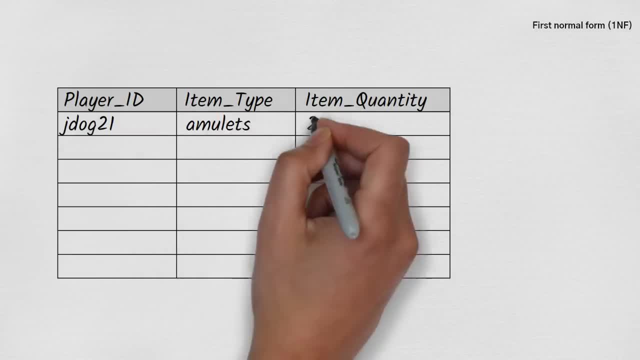 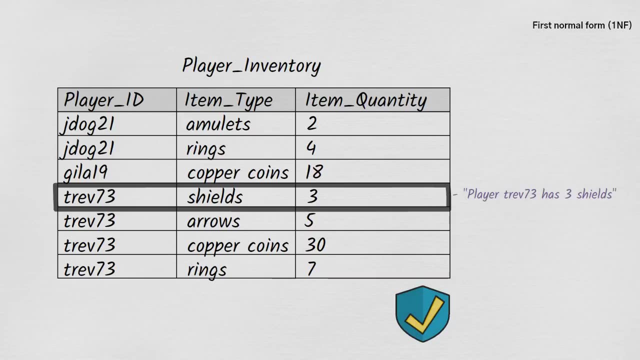 It would be this: To communicate the fact that trev73 owns three shields, we have a row for player trev73. item type: shields. item quantity: 3.. To communicate the fact that trev73 also owns two shields, we have a row for player item. 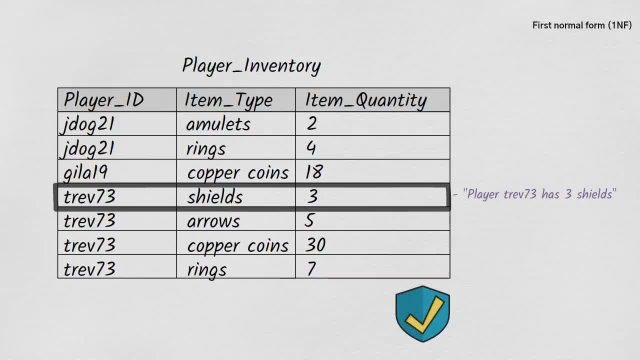 73 also owns 5 arrows. we have a row for player trev 73, item type: arrows, item quantity 5, and so on, And because each row in the table tells us about one unique combination of player and item type, the primary key is the combination of player and item type. 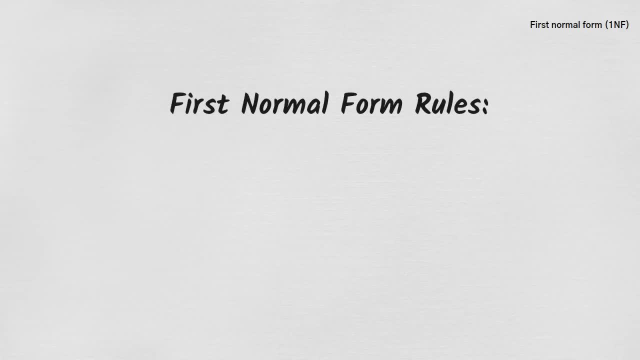 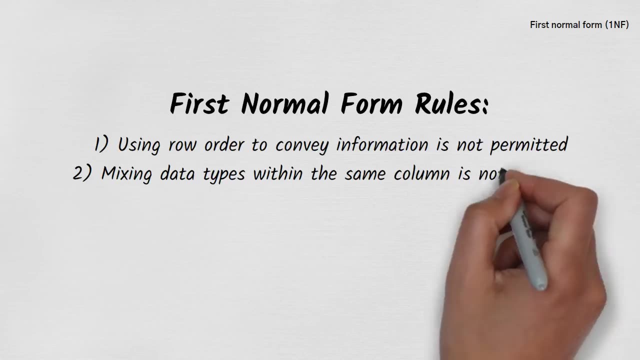 So let's review what we know about. first, normal form. Number one: using row order to convey information is not permitted. Number two: mixing data types within the same column is not permitted. Number three: having a table without a primary key is not permitted. 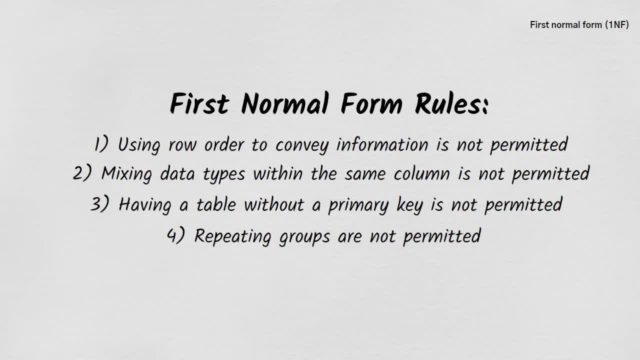 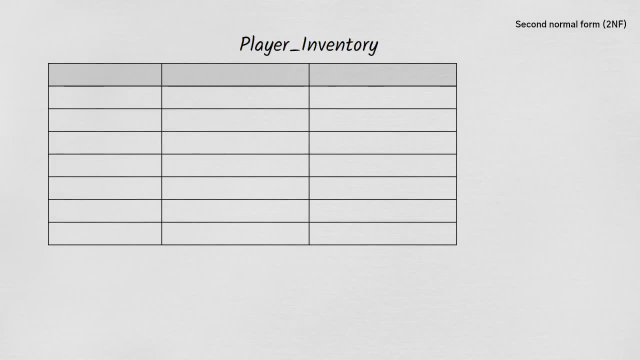 And number four repeating groups are not permitted. Next up, second normal form: Let's look again at our player inventory table. This table is fully normalized, but suppose we enhance the table slightly. Let's imagine that every player has a rating: beginner, intermediate or advanced. 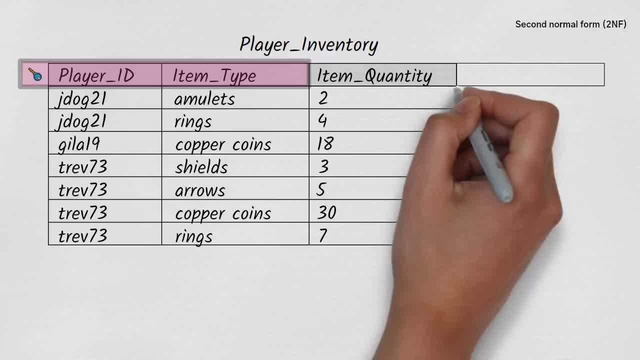 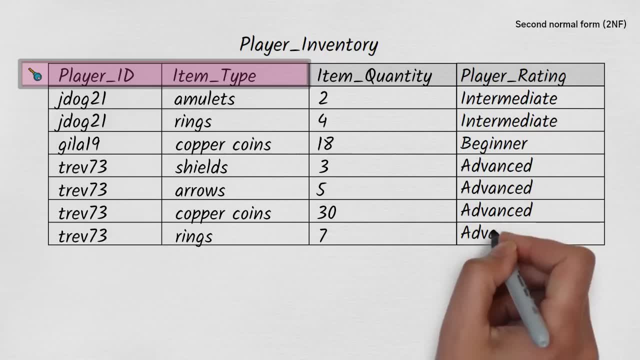 We want to record the current rating of each player and to achieve that, we simply include in our table an extra column called player rating. Notice what's happening here. Player jdog 21 has a player rating of intermediate, but because jdog 21 has two rows in the table, 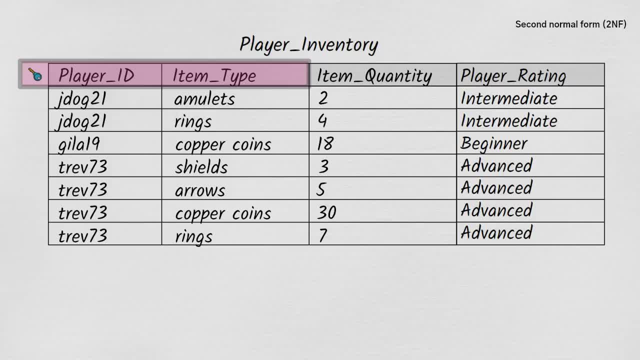 both those rows have to be marked intermediate. Player trev 73 has a player rating of advanced, but because trev 73 has four rows in the table, all four of those rows have to be marked advanced. This is not a good design. 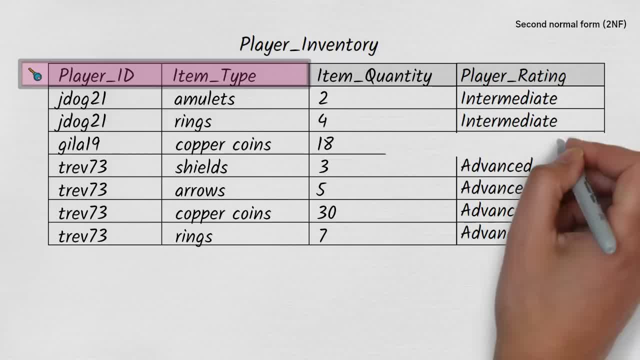 Why not? Well, suppose player gila 19 loses all her copper coins, leaving her with nothing in her inventory. The single entry that she did have in the player inventory table is now gone. If we try to query the database to find out what gila 19's player rating is, we're out. 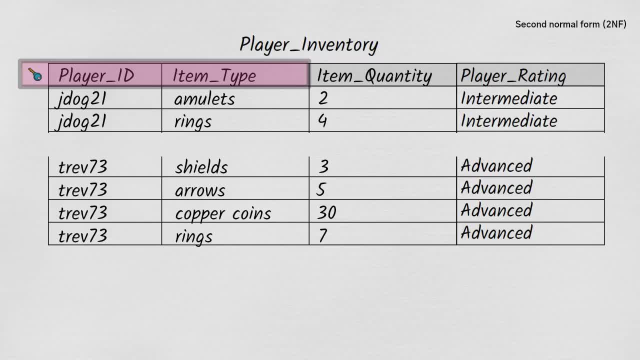 of luck. We can no longer access gila 19's player rating because the database no longer knows what the player rating is. The player no longer knows it. This problem is known as a deletion anomaly. And that's not all. Suppose jdog 21 improves his rating from intermediate to advanced. 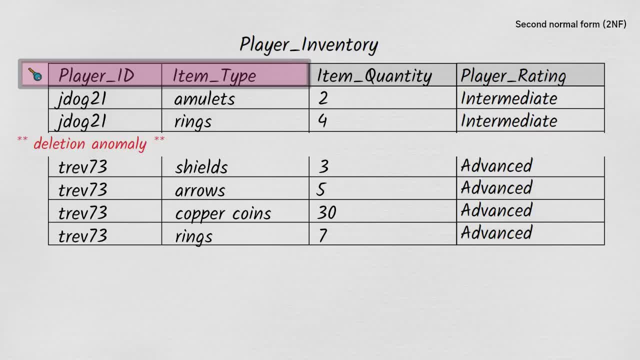 To capture his new advanced rating in the player inventory table. we run an update on his two records, But let's imagine the update goes wrong By accident. only one of jdog 21's records gets updated and the other record gets left. 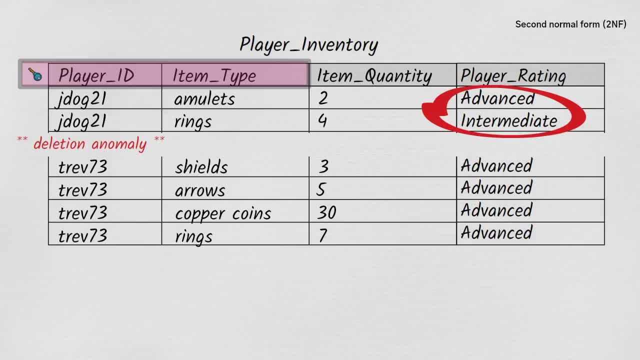 alone. Now the data looks like this: As far as the database is concerned, jdog 21 is somehow both intermediate and advanced at the same time. Our table design has left the door open for this type of logical inconsistency. This problem is called an update anomaly. 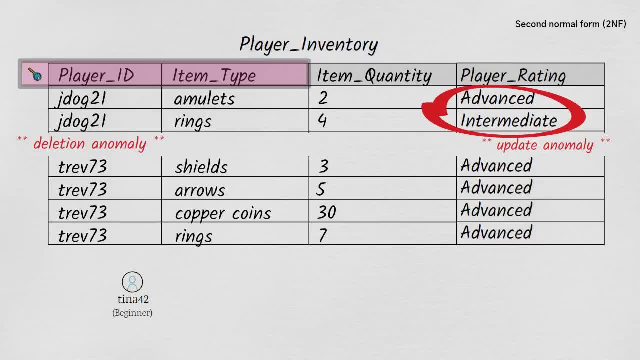 Or suppose a new player called tina 42 comes along. She's a beginner and she doesn't have anything in her inventory yet We want to record the fact that she's a beginner, but because she has nothing in her inventory we can't insert a tina 42 row into the player inventory table. 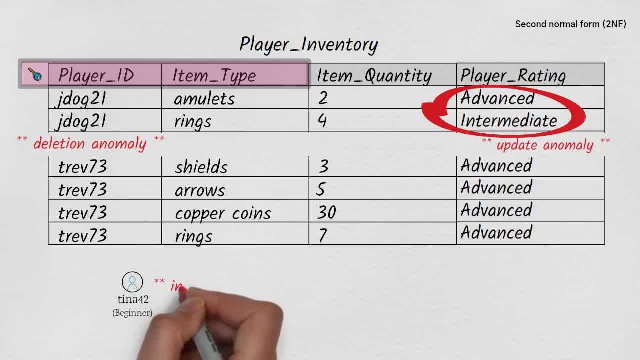 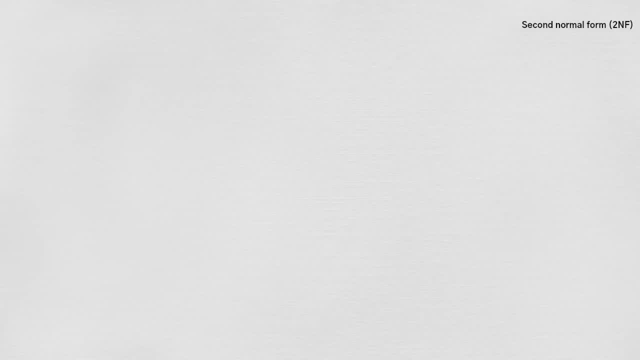 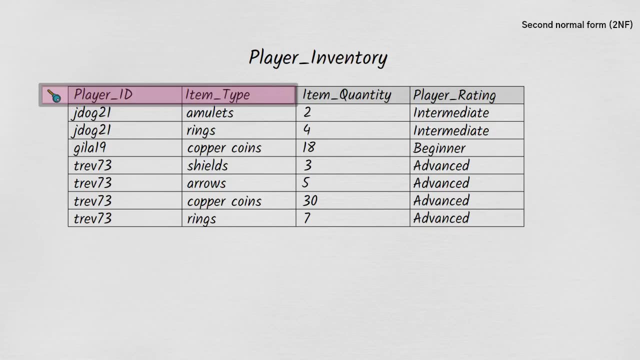 So her rating goes unrecorded. This problem is known as an insertion anomaly. The reason our design is vulnerable to these problems is that it isn't in second normal form. Why not? What is second normal form? Second normal form is about how a table's non-key columns relate to the primary key. 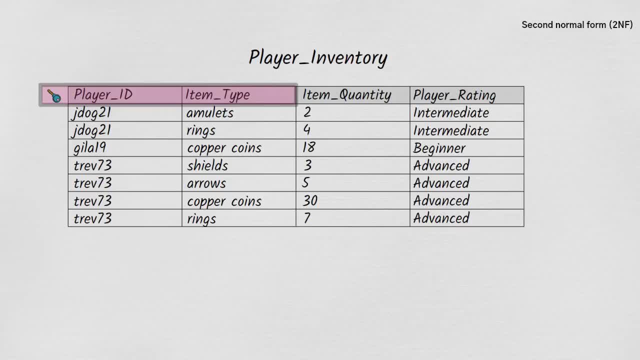 In our table, the non-key columns or, to use a slightly different terminology, non-key columns, are the non-key columns, The non-key attributes are item quantity and player rating. They are columns also called attributes that don't belong to the primary key. 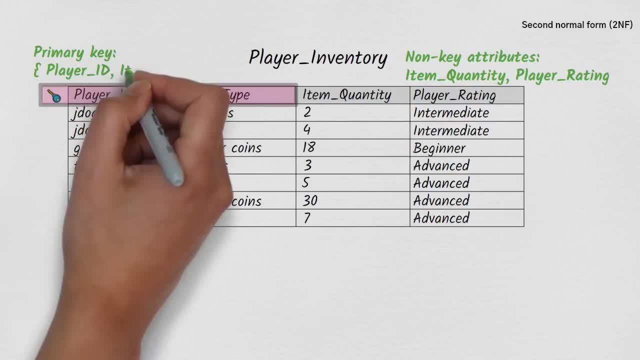 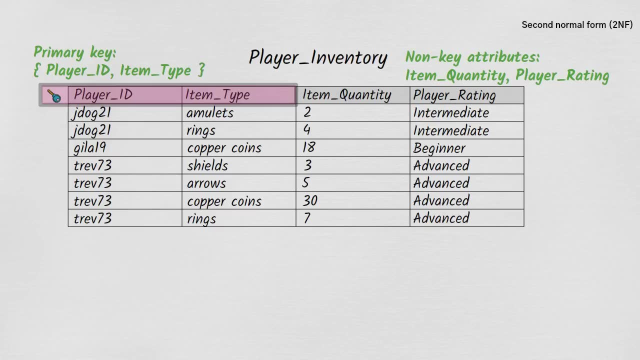 As we saw earlier, the primary key is the combination of player and item type. Now we're in a position to give a definition of second normal form. The definition we're going to give is an informal one which leaves out some nuances, but for 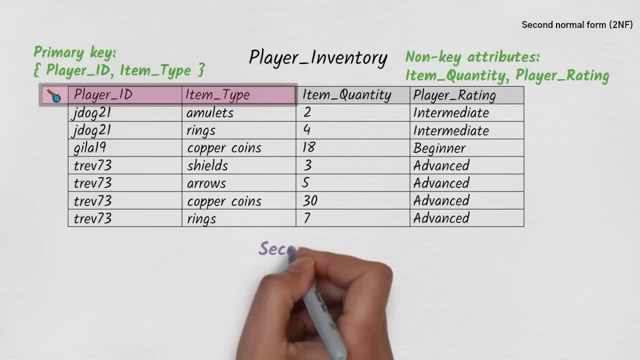 most practical purposes that shouldn't matter Informally. what second normal form says? It says that each non-key attribute in the table must be dependent on the entire primary key. How does our table measure up to this definition? Let's examine our non-key attributes, which are the attributes item, quantity and player. 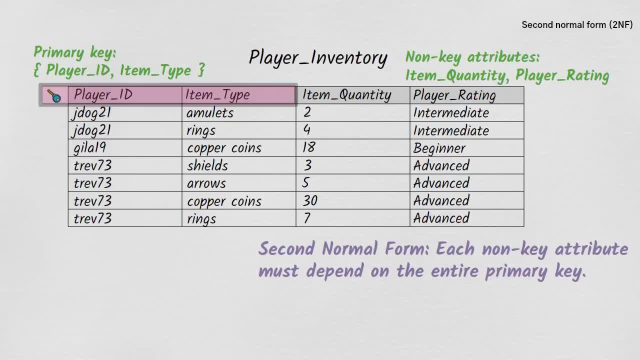 rating. Does item quantity depend on the entire primary key? Yes, because an item quantity is about a specific item type owned by a specific player. We can express it like this: The arrow signifies a dependency, or to give it its proper name, 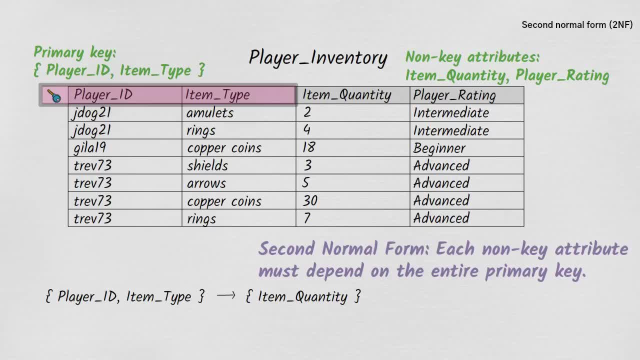 A functional dependency. This simply means that each value of the thing on the left side of the arrow is associated with exactly one value of the thing on the right side of the arrow. Each combination of player ID and item type is associated with a specific value of item. 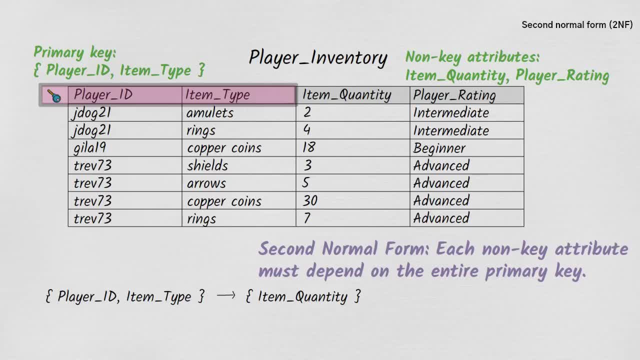 quantity. For example, the combination of player ID jdog21 and item type amulets- is associated with an item quantity of 2.. As far as second normal form is concerned, this dependency is fine because it's a dependency on the entire primary key. 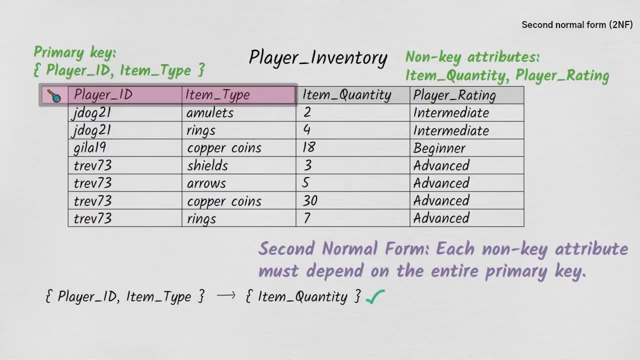 But what about the other dependency? Does player rating depend on the entire primary key? No, it doesn't. Player rating is a property of the player only. In other words, for any given player there's one player rating. This dependency on player is the problem. 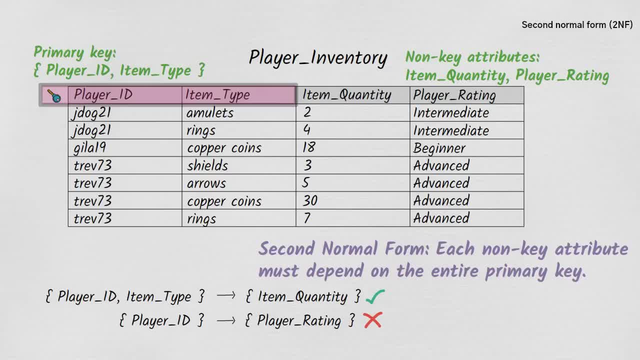 It's a problem because player isn't the primary key. Player is part of the primary key, but it's not the whole key. That's why the table isn't in second normal form And that's why it's vulnerable to problems. At what point did our design go wrong and how can we fix it? 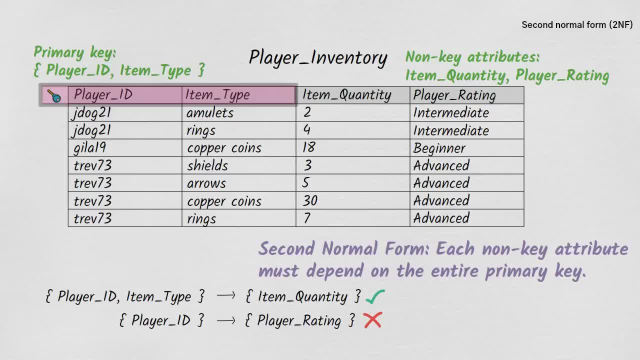 The design went wrong when we chose to add a player rating column to a table where it didn't really belong. The fact that a player rating is a property of a player should have helped us to realize that a player is an important concept in its own right, so surely a player deserves its. 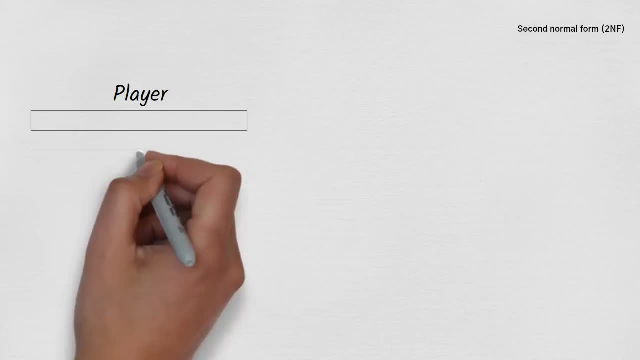 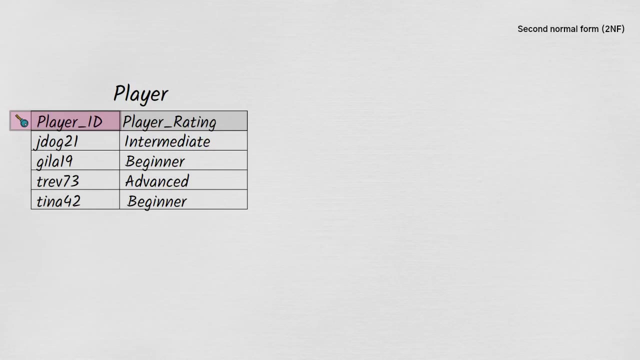 own table. Nothing could be simpler than that. A player table will contain one row per player, And in it we can include a number of players. We can include as columns the ID of the player, the rating of the player, as well as all sorts. 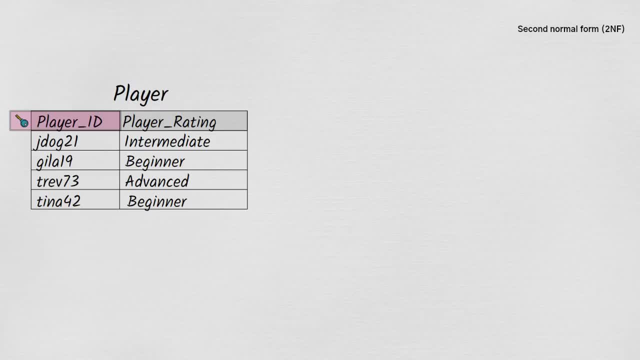 of other properties of the player. Maybe the player's date of birth, for example, Maybe the player's email address. Our other table player inventory can stay as it was. For both tables we can say that there are no part key dependencies. 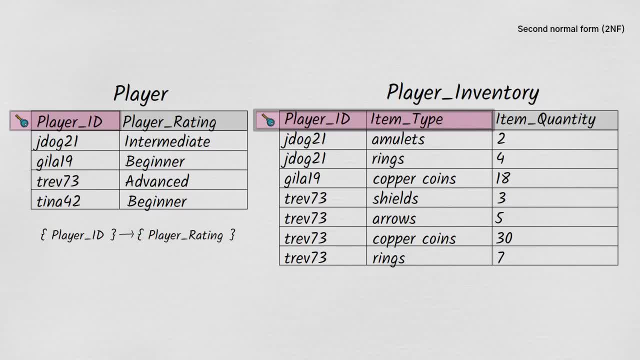 In other words, it's always the case that every attribute depends on the whole primary key, not just part of it, And so our tables are in second normal form. Now let's move on to third normal form. Suppose we decide to enhance the player table. 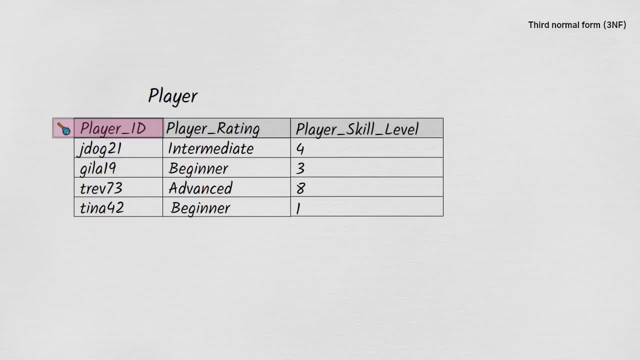 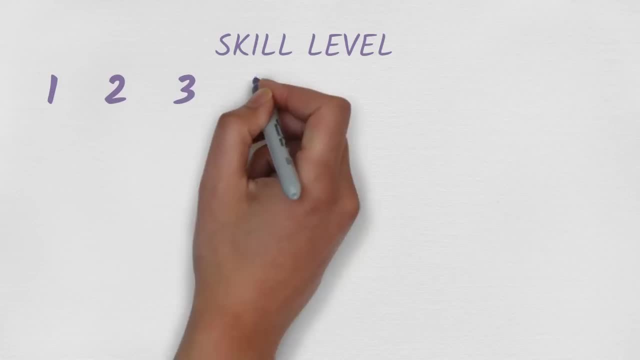 We decide to add a new column called player skill level. Imagine that in this particular multiplayer game, there's a nine point scale for skill level. At one extreme, a player with skill level one is an absolute beginner. At the opposite extreme, a player with skill level nine is as skillful as it's possible. 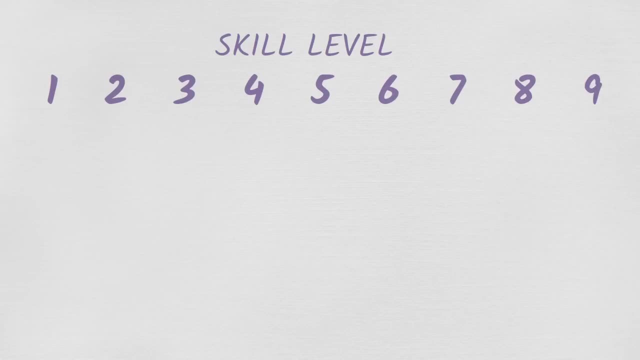 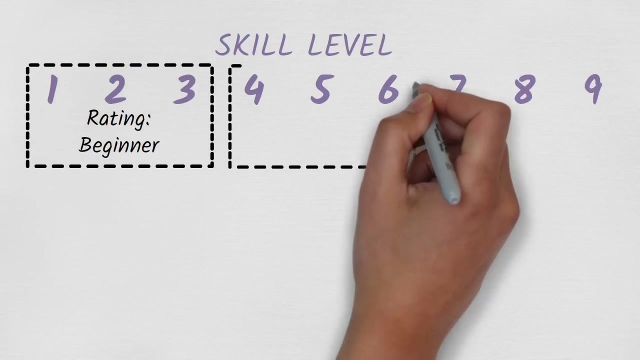 to be, And let's say that we've defined exactly how player skill levels relate to player ratings: Beginner means a skill level between one and three, intermediate means a skill level between four and six, and advanced means a skill level between seven and nine. 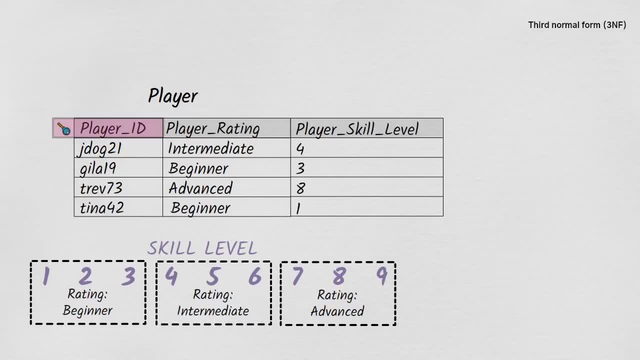 But now that both the player rating and the player skill level exist in the player table, a problem can arise. Let's say that tomorrow, player Gila 19's skill level increases from three to four. If that happens, we'll update her row in the player table to reflect this new skill level. 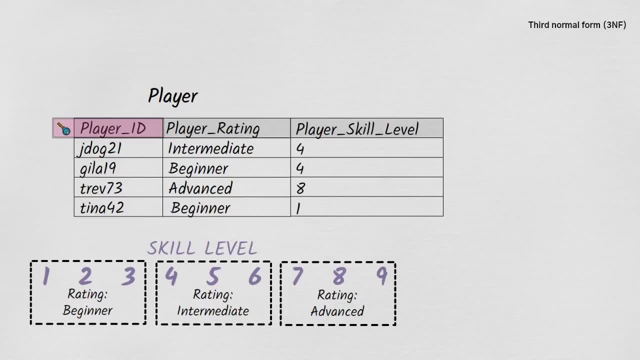 By rights we should also update her player rating to intermediate, but suppose something goes wrong and we fail to update the player rating. Now we've got a data inconsistency. Gila 19's player rating says she's a beginner, but her player skill level implies she's intermediate. 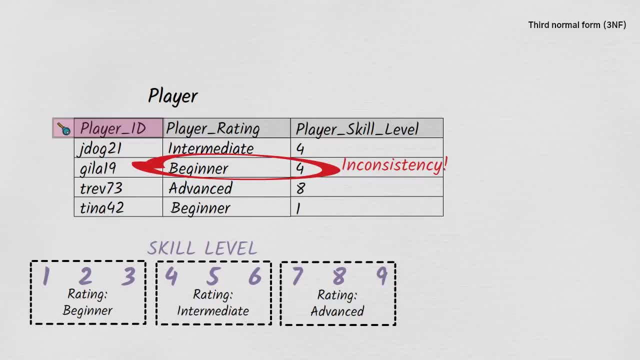 How did the design allow this to happen? Second, normal form didn't flag up any problems. There's no attribute here. that depends only partially on the primary key. As a matter of fact, the primary key doesn't have any parts, It's just a single attribute. 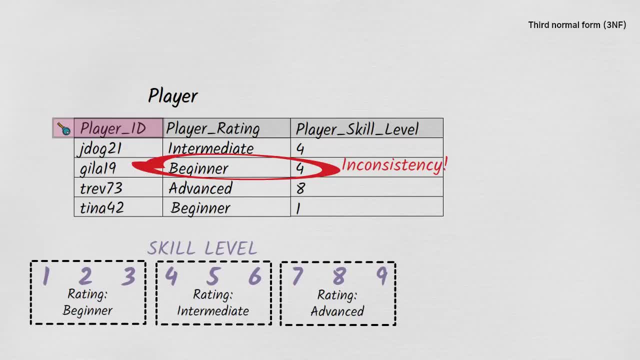 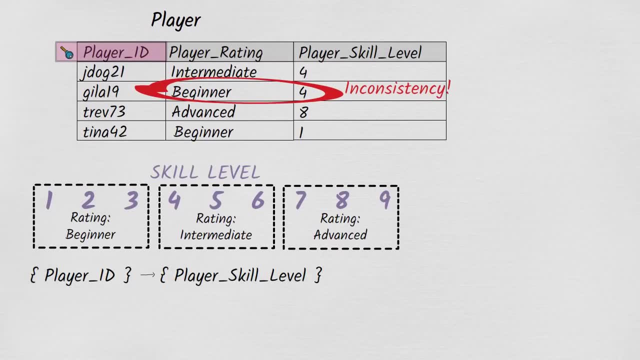 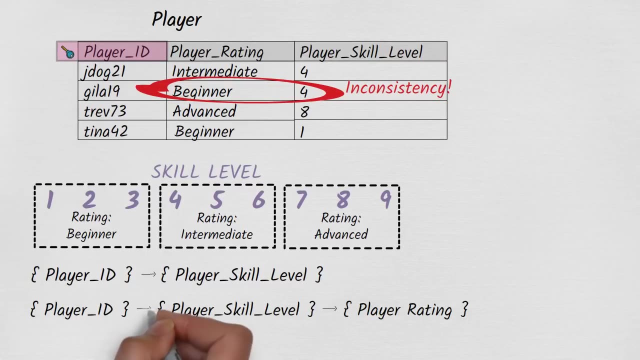 And both player rating and player skill level are dependent on it. But in what way are they dependent on it? Let's look more closely. Player skill level is dependent on player ID. Player rating is dependent on player ID too, but only indirectly, like this: 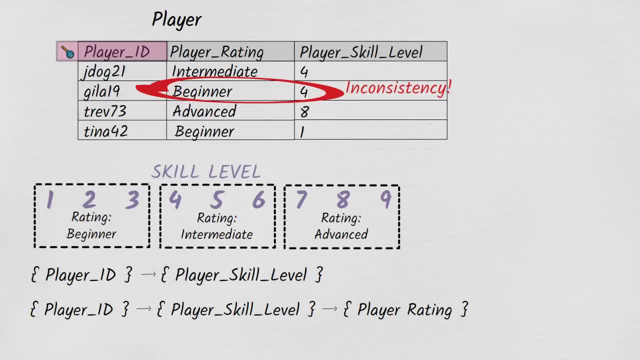 A dependency of this kind is called a transitive dependency. Player rating depends on player skill level, which in turn depends on the primary key player ID. The problem is located just here, Because what third normal form forbids is exactly this type of dependency, the dependency. 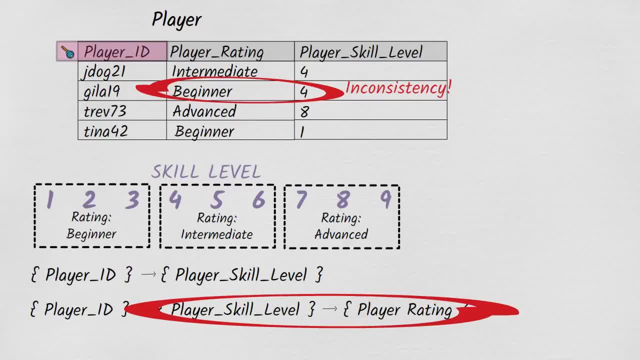 of a non-key attribute on another non-key attribute, Because player rating depends on player skill level, which is a non-key attribute. this table is not in third normal form. There's a very simple way of repairing the design to get it into third normal form. 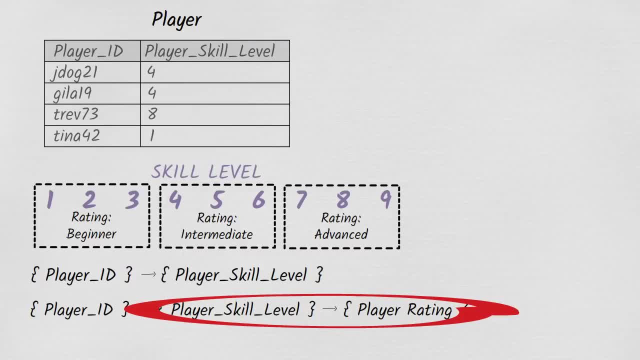 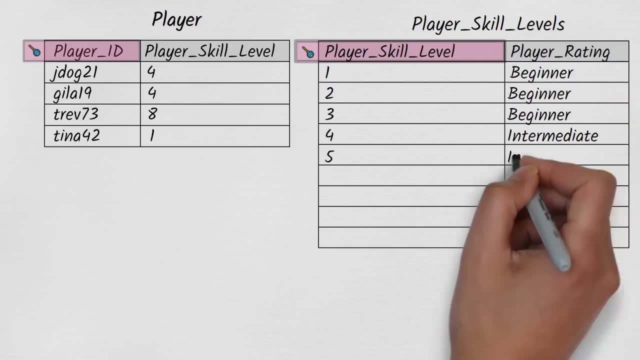 We remove player rating from the player table. So now the player table looks like this And we introduce a new table called player skill levels. The player skill levels table tells us everything we need to know about how to translate player skill level into a player rating. 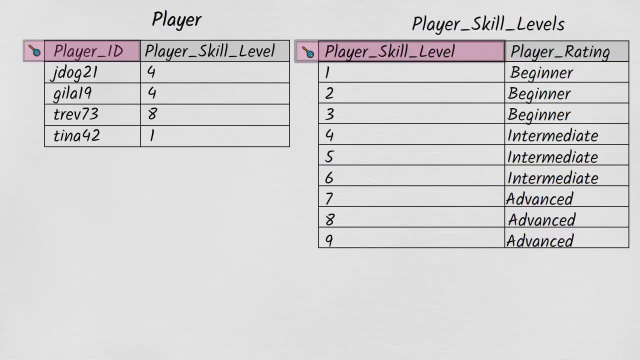 Third, normal form is the culmination of everything we've covered about database normalization so far. It can be summarized in this way: Every non-key attribute in a table should depend on the key, the whole key and nothing but the key. If you commit this to memory and connect the key to the non-key attribute, you can get: 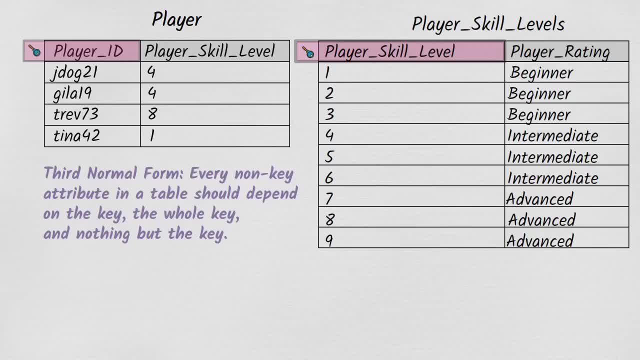 a non-key attribute. If you keep it constantly in mind while you're designing a database, then 99% of the time you will end up with fully normalized tables. It's even possible to shorten this guideline slightly by knocking out the phrase non-key. 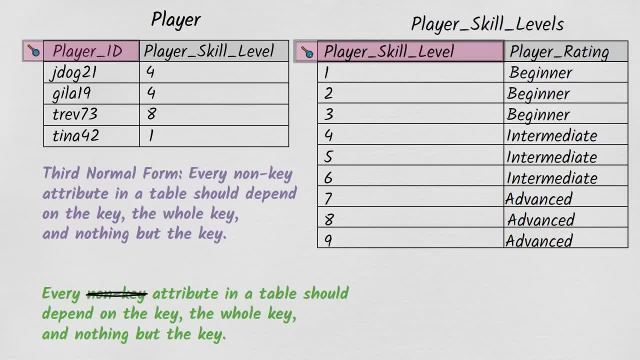 giving us the revised guideline. every attribute in a table should depend on the key, the whole key and nothing but the key, And this new guideline represents a slightly stronger flavor of third normal form, known as Boyce-Codd normal form. This means that a table with Boyce-Codd normal form is extremely small and the chances of 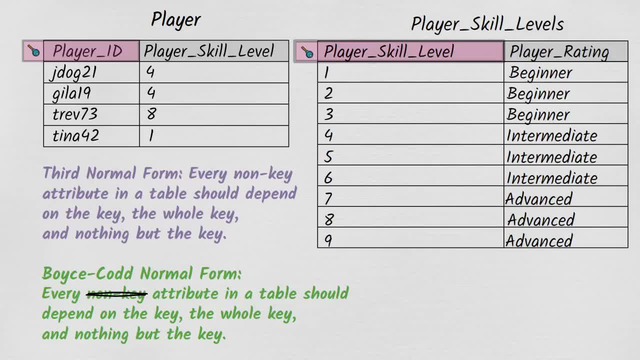 you ever encountering a real-life third normal form table that doesn't meet Boyce-Codd normal form are almost zero. Any such table would have to have what we call multiple overlapping candidate keys, which gets us into realms of obscurity and theoretical rigor that are a little beyond. 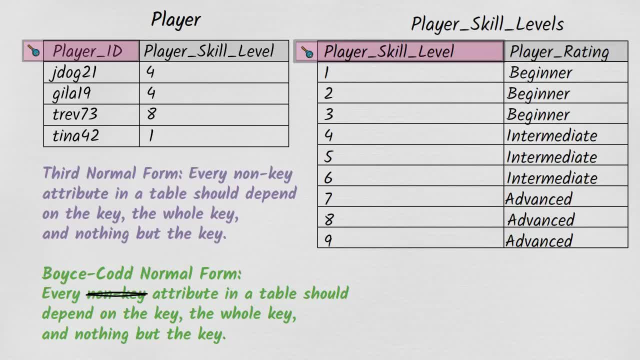 the scope of this video. So, as a practical matter, just follow the guideline that every attribute in a table should depend on the key, the whole key and nothing but the key, the whole key and nothing but the key, and you can be confident that the table will be in both third normal form. 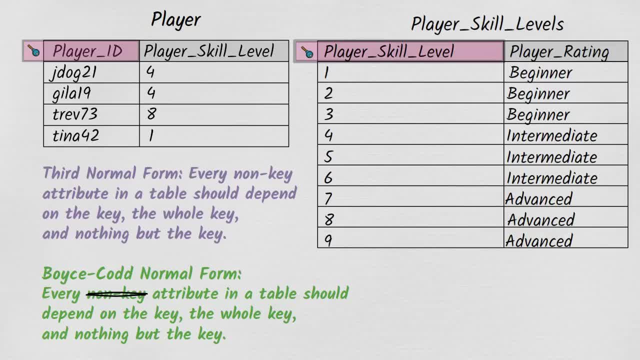 and Boyce-Codd normal form. In almost all cases, once you've normalized a table this far, you've fully normalized it. There are some instances where this level of normalization isn't enough. These rare instances are dealt with by fourth and fifth normal form. 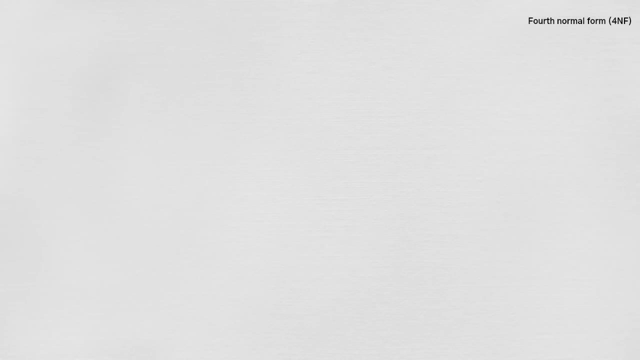 So let's move on to fourth normal form. We'll look at an example of a situation where third normal form is the most common form of a table. Third normal form isn't quite good enough and something a bit stronger is needed. In our example, there's a website called designmybirdhousecom, the world's leading supplier of customized 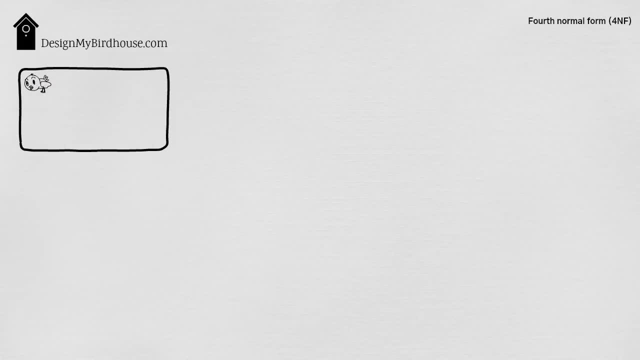 birdhouses On designmybirdhousecom. customers can choose from different birdhouse models and for the model they've selected, they can choose both a custom color and a custom style. Each model has its own range of available colors and styles. 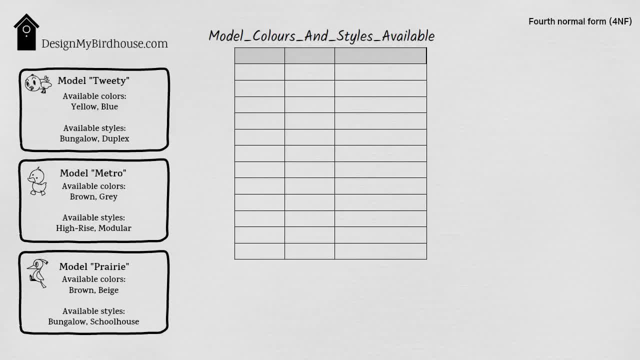 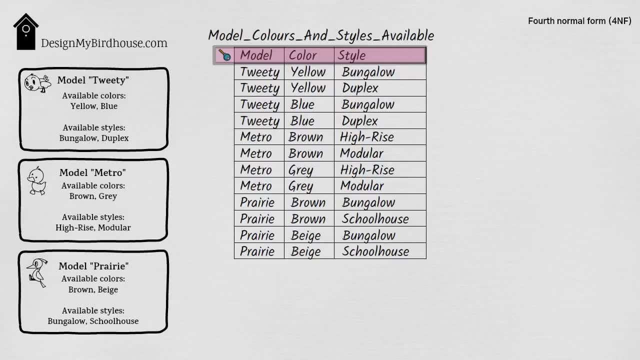 One way of capturing this information is to put all the possible colors and styles together. Another way is to put all the possible combinations in a single table like this. This table is in third normal form. The primary key consists of all three columns: model, color and style. 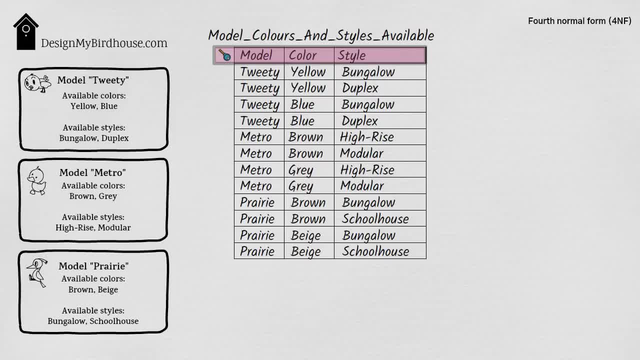 Everything depends on the key, the whole key and nothing but the key. And yet this table is still vulnerable to problems. Let's look at the rows for the birdhouse model prairie. The available colors for the prairie birdhouse model are brown and beige. 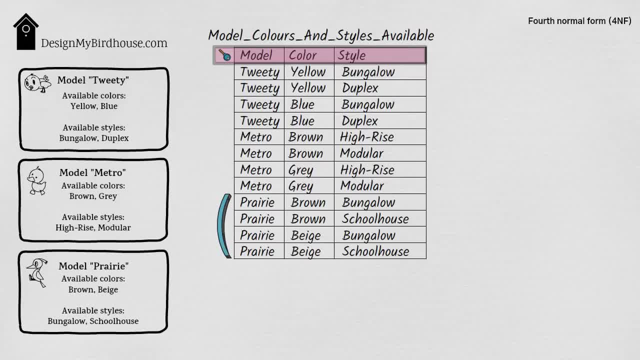 Now suppose designmybirdhousecom decides to introduce a third available color for the prairie model: green. This will mean we'll have to add two extra prairie rows to the table, one for green bungalow and one for green schoolhouse. 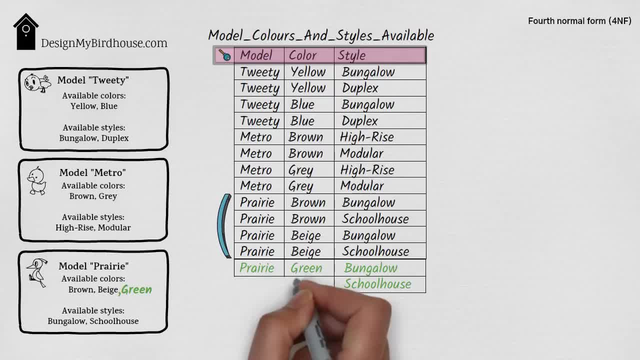 If, by mistake, we only add a row for green bungalow and fail to add the row for green schoolhouse, then we have a data inconsistency. Available colors are supposed to be completely independent of available colors. So if we add a row for green bungalow and fail to add the row for green schoolhouse, 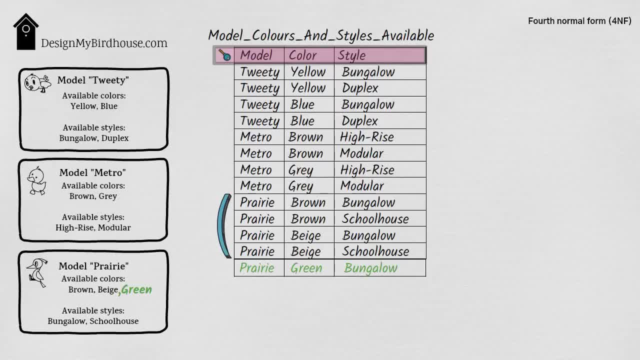 then we have a data inconsistency. But our table is saying that a customer can choose green only for the bungalow style, not for the schoolhouse style. That makes no sense. The prairie birdhouse model is available in green, so all its styles should be available. 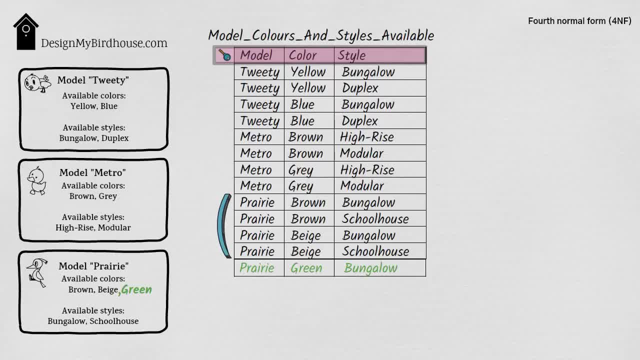 in green. Something about the way the table is designed has allowed us to represent an impossible situation. To see what's gone wrong, let's have a closer look at the dependencies among models, colors and styles. Can we say that color has a functional dependency on green? 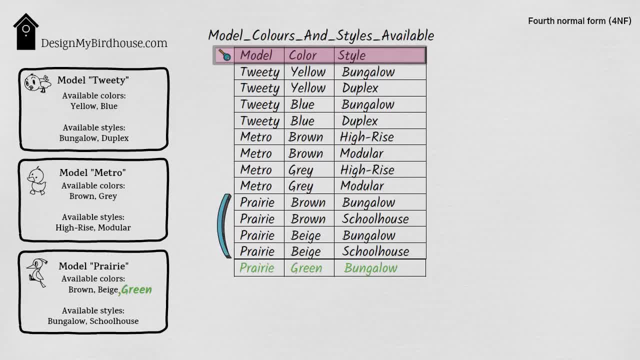 Actually no, because a specific model isn't associated with just one color, And yet it does feel as though color has some relationship to model. How can we express it? We can say that each model has a specific set of available colors. 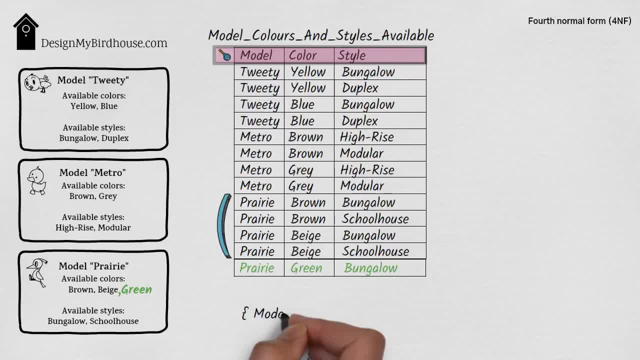 This kind of dependency is called a multi-valued dependency, and we express it with a double headed arrow like this: And it's equally true that each model has a specific set of available colors. This is called a multi-valued dependency, And we express it with a double-headed arrow like this: 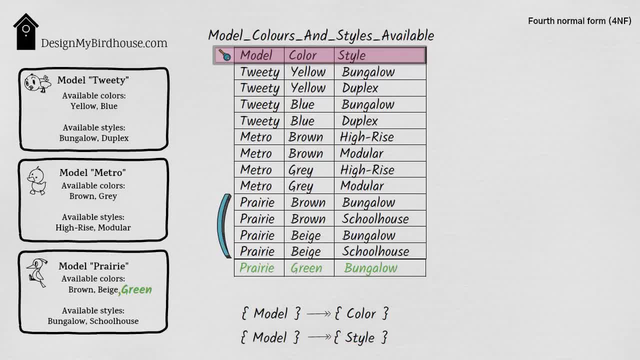 has a specific set of available styles. What fourth normal form says is that the only kinds of multi-value dependency we're allowed to have in a table are multi-value dependencies on the key. Model is not the key, so the table model colors and styles available is not in fourth normal form. 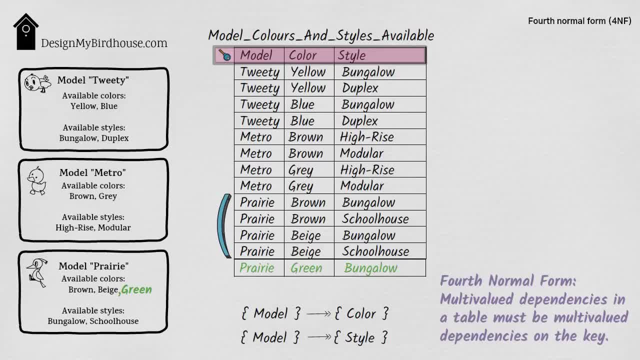 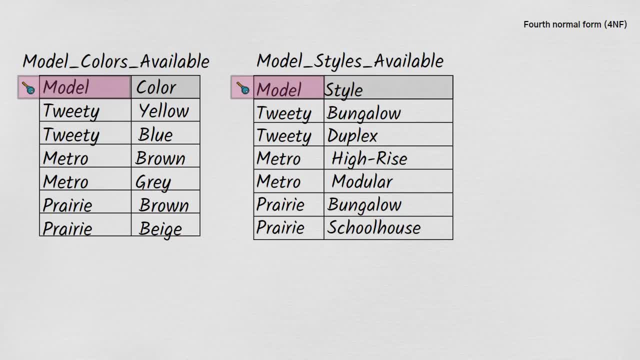 As always, the fix is to split things out into multiple tables. Now, if designmy birdhousecom expands the range of prairie model colors to include green, we simply add a row to the model colors available table and no anomalies are possible. 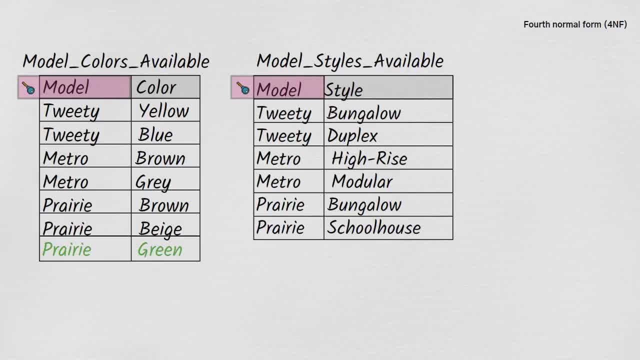 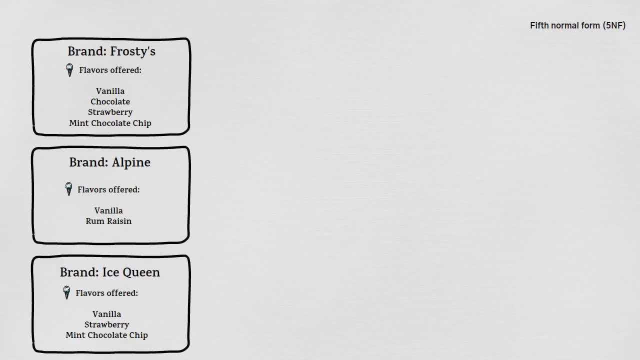 We're now ready for fifth normal form, the last normal form covered in this video. As our fifth normal form example, we imagine that there are three different brands of ice cream available: Frosties, Alpine and Ice Queen. Each of the three brands of ice 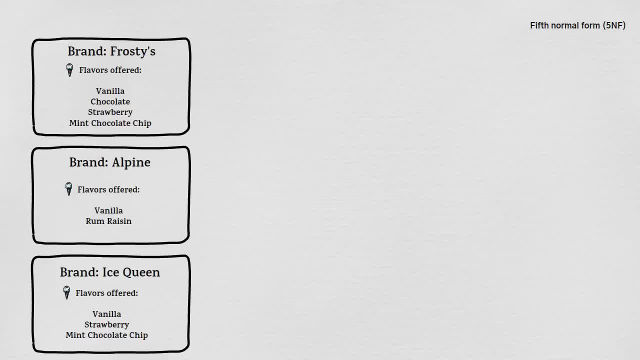 cream offers a different range of flavors: Frosties offers vanilla, chocolate, strawberry and mint chocolate chip, Alpine offers vanilla and rum raisin, and Ice Queen offers vanilla, strawberry and mint chocolate chip. Now we ask our friend Jason what types of ice cream he likes, Jason says: I only like vanilla and 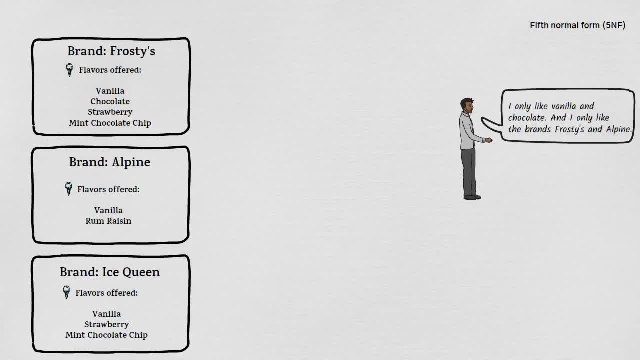 chocolate and I only like the brands Frosty and Alpine. We ask our other friend, Susie, what types of ice cream she likes. Susie says: I only like rum, raisin, mint, chocolate chip and strawberry and I only like the brands Alpine and Ice Queen. So after a little bit of brain work, we 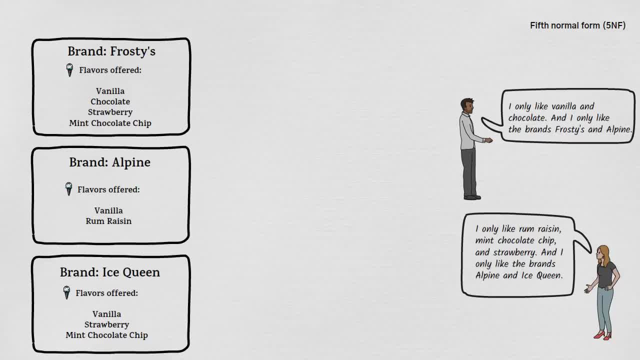 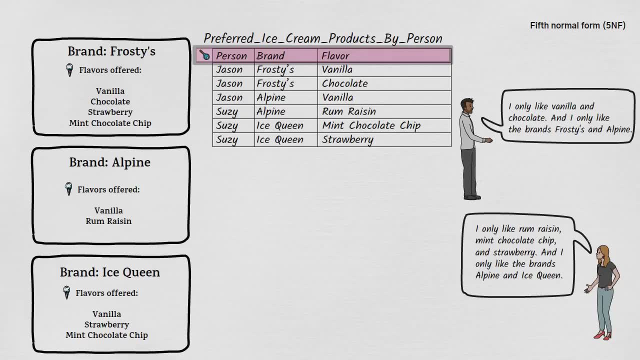 deduce exactly which ice cream products Jason and Susie are willing to eat, and we express this in a table. But time passes, tastes change and at some point Susie announces that she now likes Frosty's brand ice cream too, So we need. 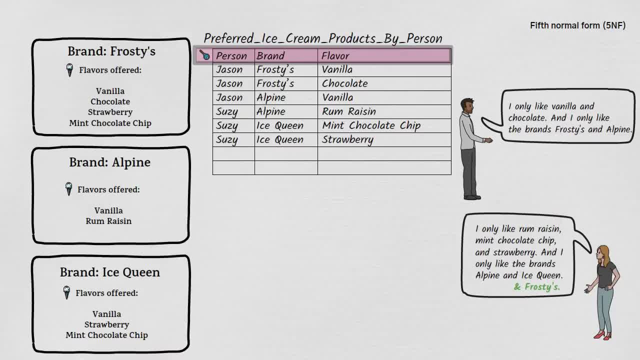 to update our table. It won't come as any surprise that we might get this update wrong. We might successfully add a row for person Susie brand Frosty's flavor strawberry, but fail to add a row for person Susie brand Frosty's flavor mint chocolate chip. And this outcome wouldn't just 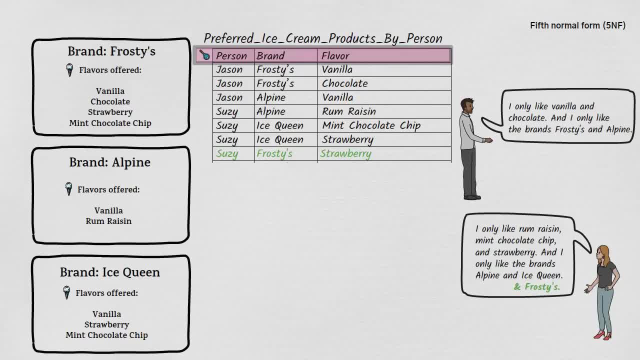 be wrong. it would be logically inconsistent because we've already established that Susie likes Frosty's brand and likes mint chocolate chip flavor and therefore there's no way she can dislike it. So we need to add a row for person: Susie, brand, Frosty's flavor, mint chocolate chip. 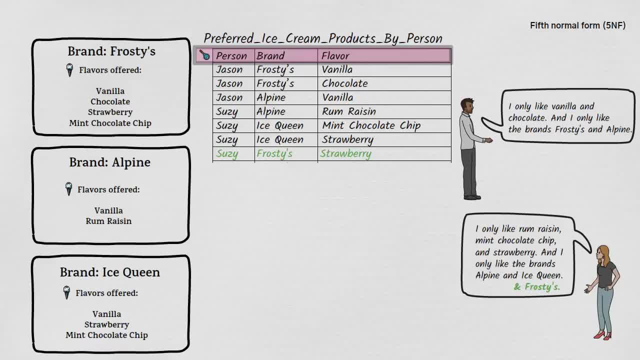 In this example, we went wrong right at the beginning. At the beginning, we were given three pieces of information. First, we were told which brands offered which flavors. Second, we were told which people liked which brands. Third, we were told which people liked which. 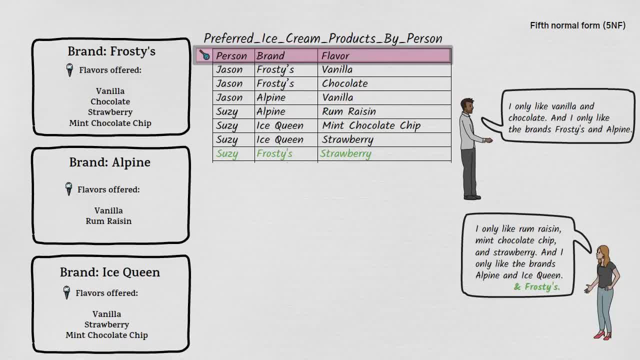 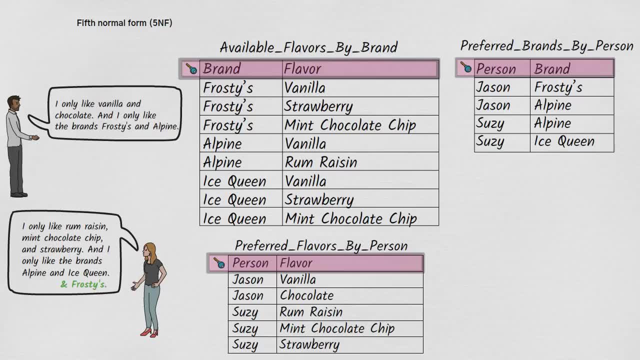 flavors. From those three pieces of information, we should have simply created three tables, And that's all we needed to do. All the facts of the situation have been represented. If we ever want to know what specific products everyone likes, we can simply ask the database. 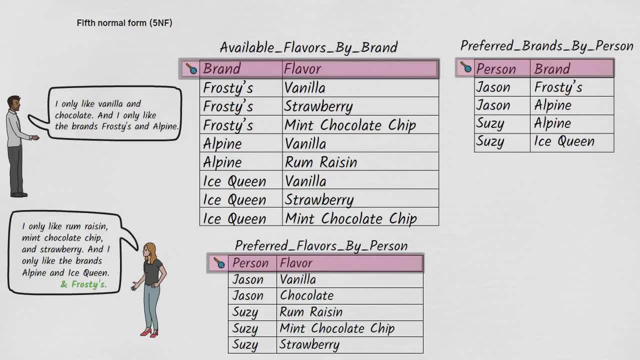 platform expressing our question in the form of a piece of SQL that logically deduces the answer by joining the tables together. To sum things up, if we want to ensure that a table that's in fourth normal form is also in fifth normal form, we need to ask ourselves: 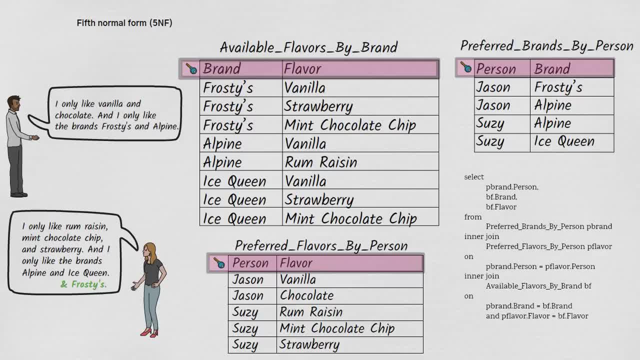 whether the table can be logically thought of. in the same way, If we want to ensure that a table that's in fourth normal form is also in fifth normal form, we need to ask ourselves whether the table can be logically thought of as being the result of joining some other. 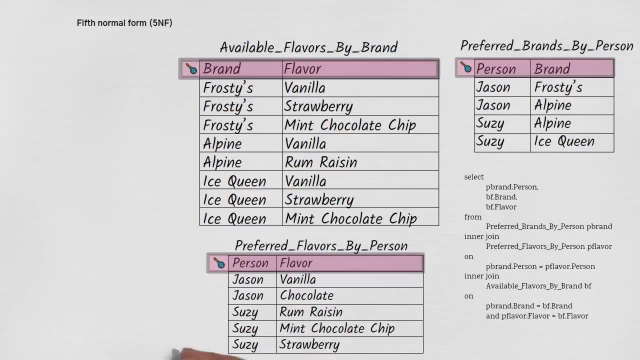 tables together. If it can be thought of that way, then it's not in fifth normal form. If it can't be thought of that way, then it is in fifth normal form. We've now covered all the normal forms, from first normal form to fifth normal form. Let's 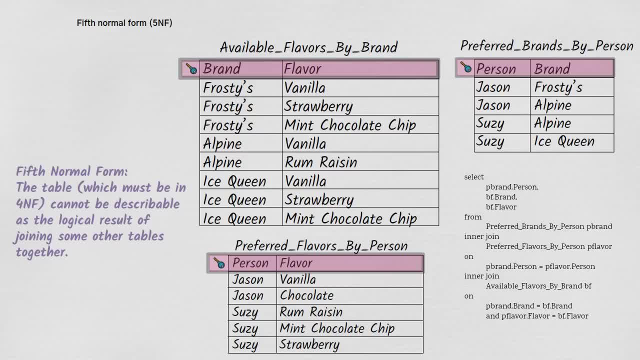 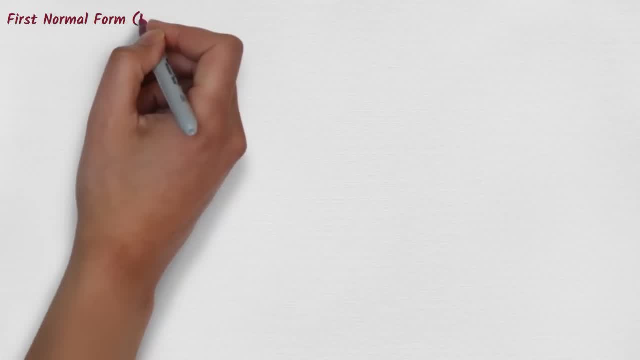 review, keeping in mind that for a table to comply with a particular normal form, it must comply with all of the lower normal forms as well. The rules for first normal form are: 1. Using row order to convey information is not permitted. 2.